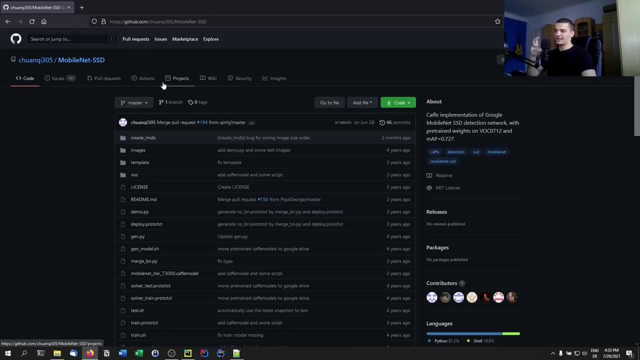 and a proto txt file from here that we're going to then use in python using opencv, to do the object recognition. Now, there are many ways to do this, but i'm going to show you how to do it, So let's get started. So there are many ways to do that. you can use yolo, you can use different models and 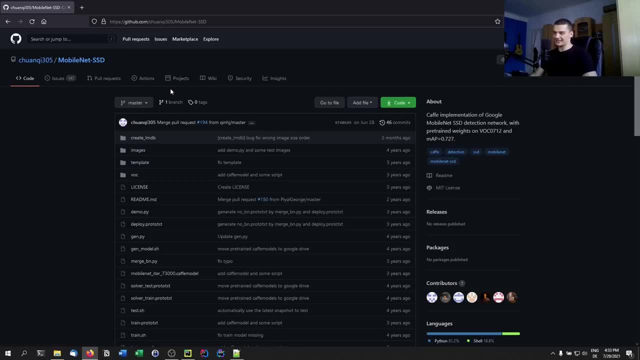 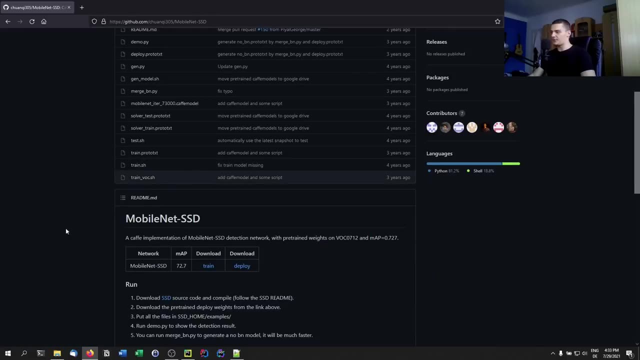 algorithms and procedures. we're going to do it like that in this video. maybe we're going to do it in another way in another video. but in order to get the model file you need to go here to the readme and in network mobilenet ssd you can go to download, deploy. this is how you get the cafe model. 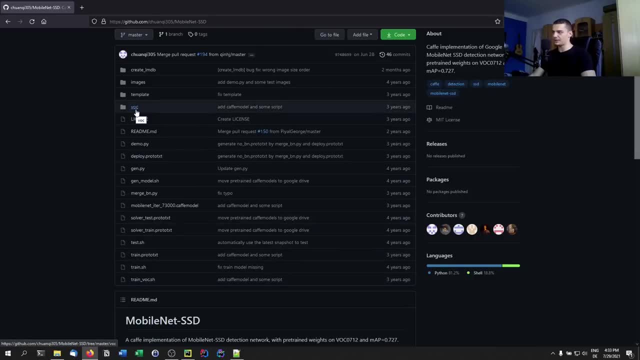 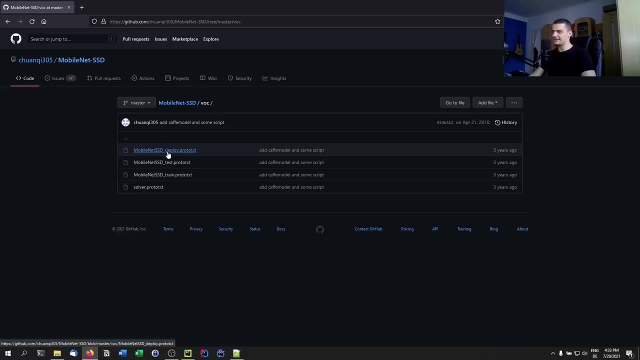 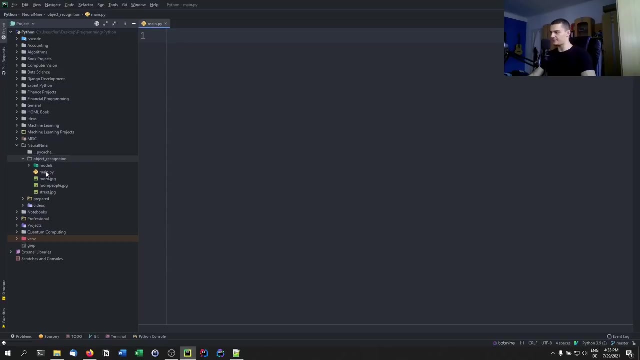 and the proto txt file is located in this directory here in voc or voc, and what you want is the mobilenet ssd deploy proto txt file. so you download these two files, you put them into your directory that you're working in, so you have this main py file. then you create, if you want to, a directory called models and 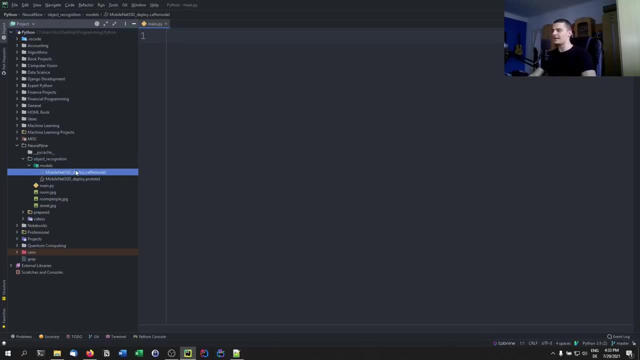 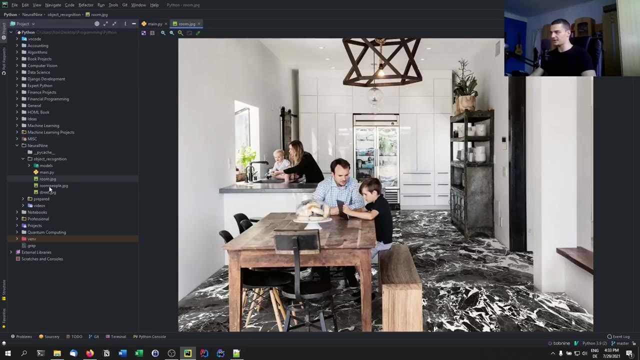 inside of it you have those two files, so you have the cafe model and you have the proto txt files. in addition to that, i also have a bunch of images here. you can choose whatever images you like. i just have some images of rooms with people or streets, because we're going to recognize some. 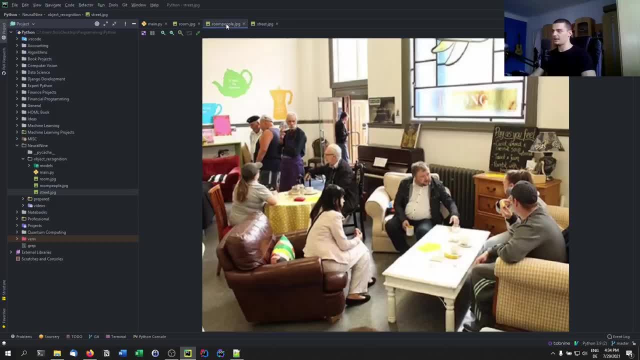 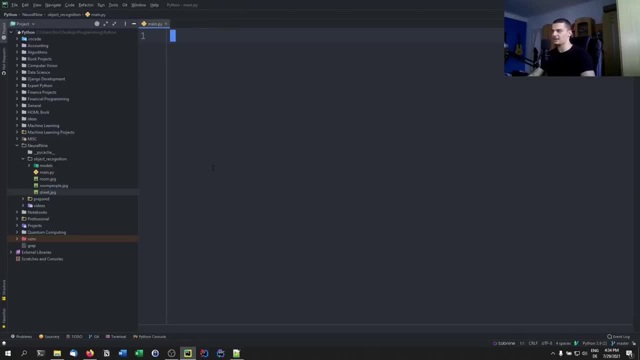 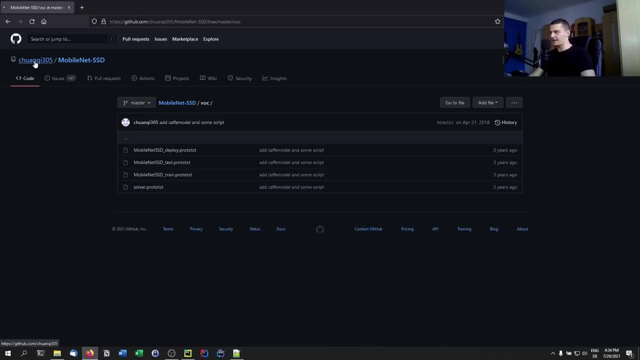 objects here, so trucks and cars and people and tables and chairs and sofas and so on. those are going to be the images. you can choose whatever images you like, but put them in the same directory. besides that, i want to mention that, of course, this code is heavily influenced by this repository here because 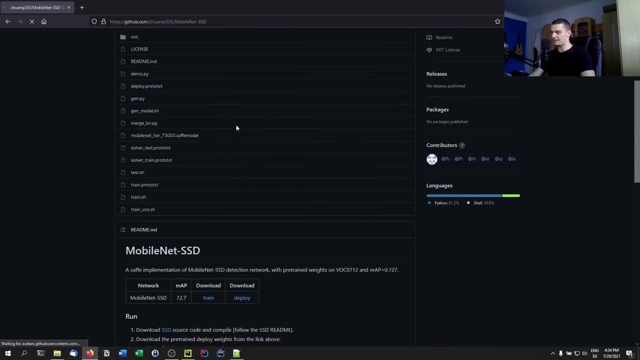 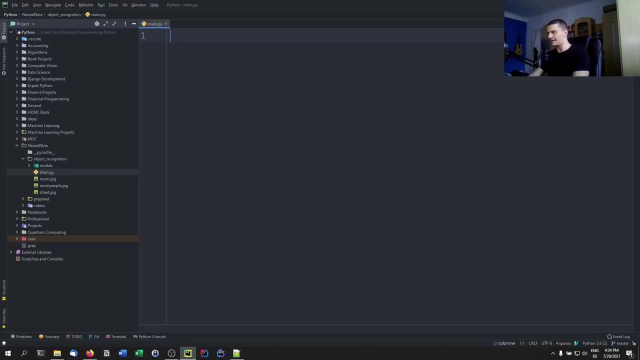 that's the guy that provided the models here, or this is where i got the models and the knowledge from, and of course also i want to mention here that i got a fair bit of inspiration from the web website pi image search- i think that's what it's called. it's called: uh, i got some of the knowledge. 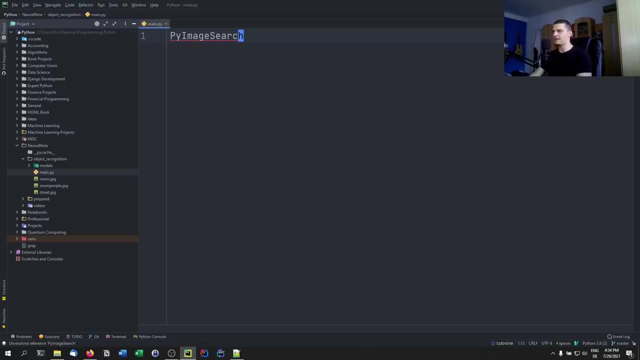 on how to use that model from that site, so i want to give credit to them. even though they were not my main source and not my only source, because i looked at a couple of different repositories and blocks- i think it's fair to give credit to them, since i uh learned how to use this um, this model. 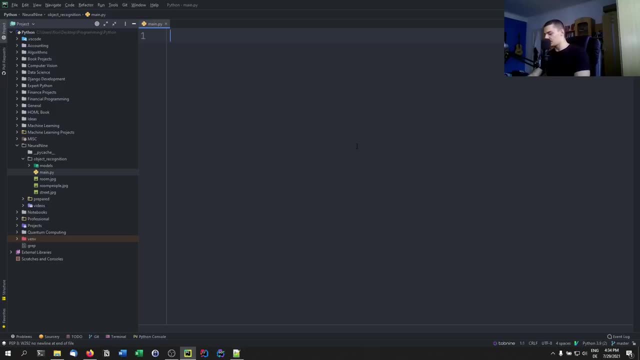 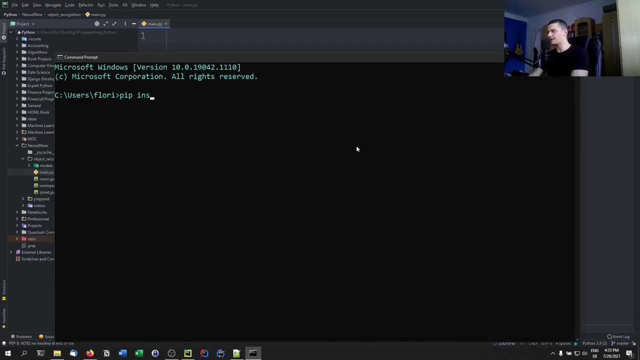 properly using their blog post. okay, so, besides that, we're going to start with opening up cmd and we're going to install the libraries we're going to need today. we're going to need numpy, so pip install numpy. uh, and we're going to need opencv, so pip install opencv-python. those are: 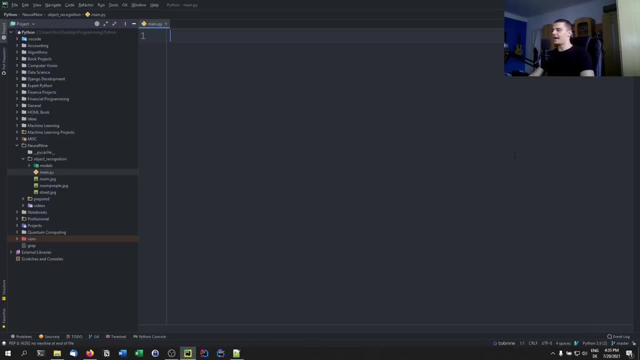 the two libraries we're going to need um and once we have installed them- i already have installed them, so i'm not going to do this again. we are going to import numpy as np and we're going to import cv2, which is opencv. even though we install opencv-python, we import cv2. 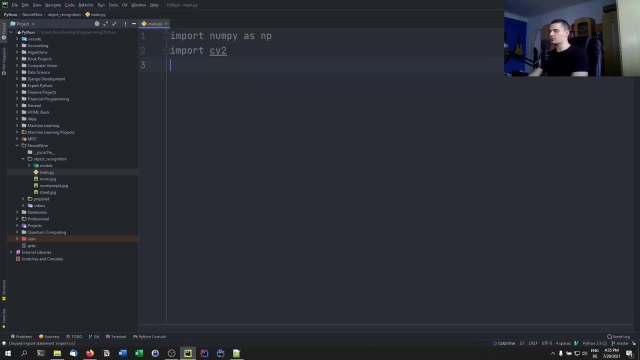 we're going to import numpy as np and we're going to import cv2, which is opencv-python. all right, so the first thing is we're going to specify all the paths to the relevant file. so we want to know, okay, where's the image that we're going to do the object recognition on. 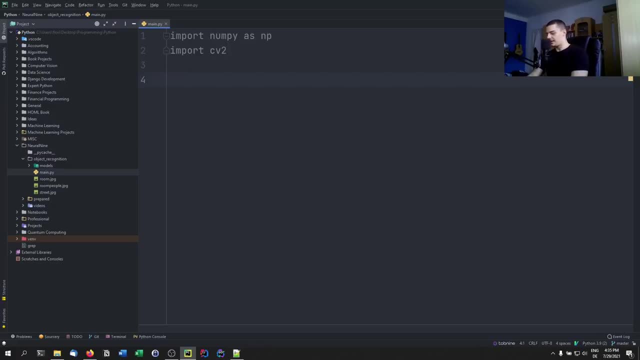 uh, where are the models? where's the proto txt file? uh, and the first thing is the image. so image path is going to be: just let's start with room people dot jpeg, then the proto txt path is going to be: models slash, and then mobilenet ssd, deploy proto txt and then the model path is going to be: 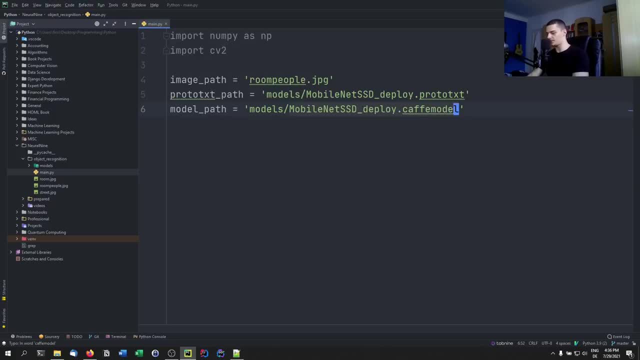 model slash mobilenet blah blah dot cafe model. uh, and we're also going to already set a parameter, because you need to think about it like that: when we detect, or when the model detects a certain object in an image, it has a certain confidence. so if it sees a chair, it can say, okay, i'm 99. 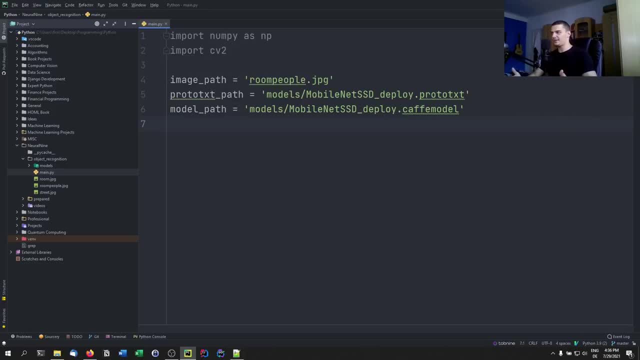 sure that this is a chair, classified as a chair. maybe it will say: i have a 15 confidence that this is going to be a chair. we need to set a minimum confidence and if this minimum confidence is not reached by the model, it's not going to do any detection, so it's not going to say: okay, this is a. 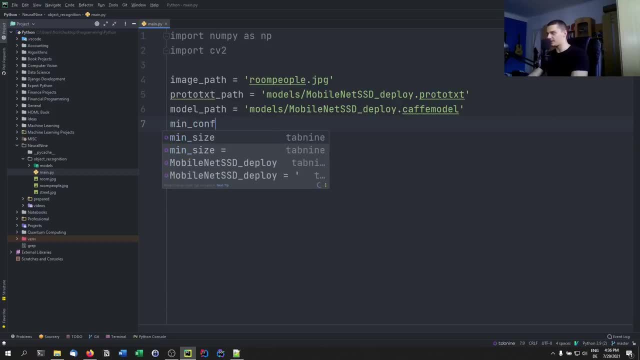 chair if it's not confident enough, and a min confidence that i think works pretty good is 20, so 0.2. um, yeah, that's basically it. next, we need to have a classes list, and this is something that, of course, you need to get from the repository. you need to know the classes for this particular module here or for this. 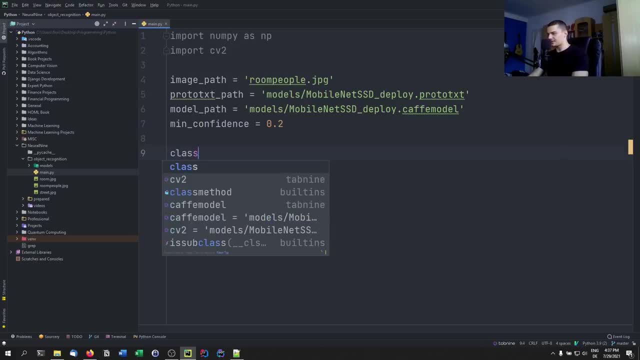 particular model here and those classes are going to be specified in the list. so we're going to have a list of classes and those are things like a background, those are things like airplane and bicycle and so on. i'm going to copy that list now. so if you want to copy it as well, you can go to. 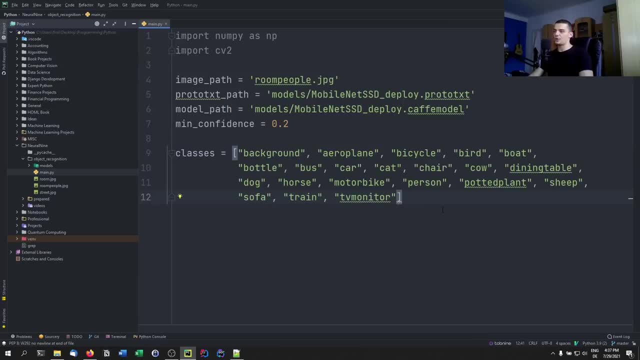 the repository and look at the individual classes. or you can just pause the video and type this code here. it's not too big, you can just copy it in the repository and look at the individual classes. big, but I don't want to waste any time in a tutorial here typing all these strings. it's not. 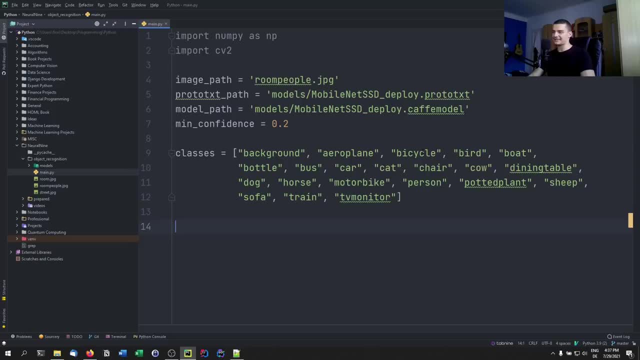 really educational. so we're going to skip that. those are all the classes that we're going to be able to classify. so birds, cows, cats, person, motorbike, train, tv monitor and so on, those are the things, and now we're going to start with the model. so before we actually, before we actually 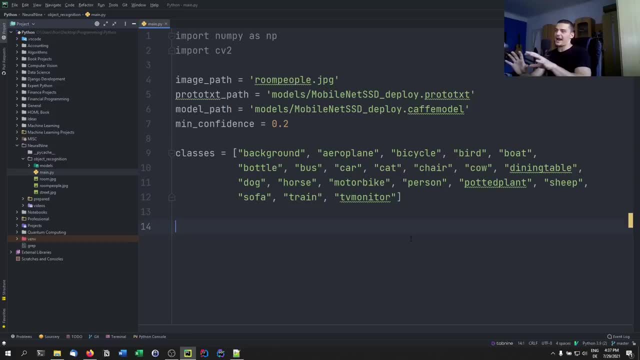 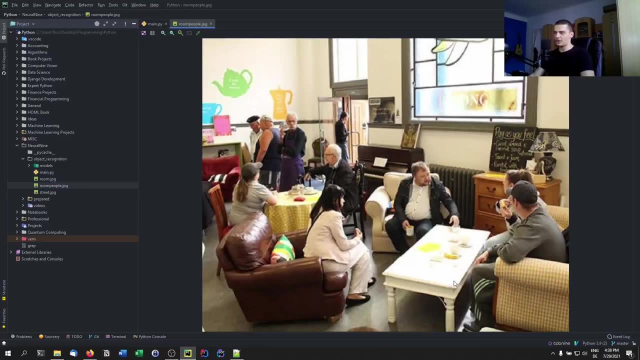 import a model, we also need to think a little bit about how are we going to then display later on that we detect as an object. and what we're going to do is we're just going to say, if the model detects this guy as a person, it's going to just put a rect angle around him. so it's going to say: 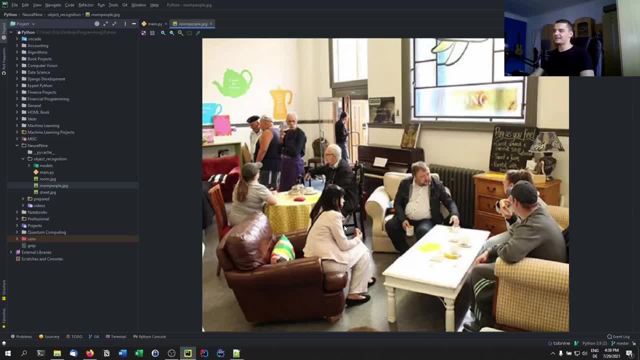 okay, this here, this area, is a person and if we have a bunch of people, we want to have the same color of the red angle. so let's say all the people are classified as blue, for example. if we want to have that, we want to have a specific color. then again, if we classify this as a sofa, we want it. 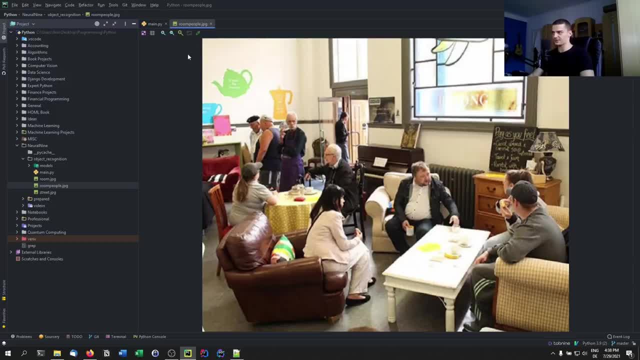 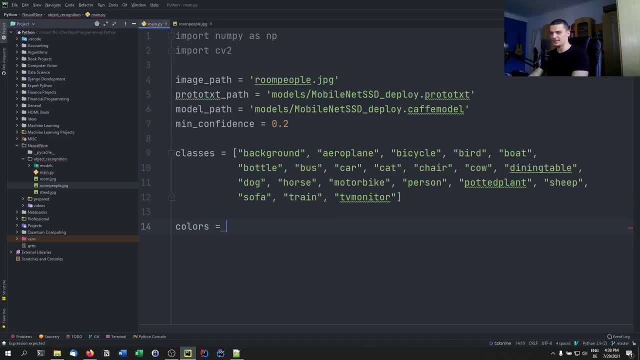 to not be blue but something else, for example green or red or something else. and in order to have random colors, we're going to generate a colors list by saying colors equals and then nprandomuniform, and we're going to generate values from 0 to 255. 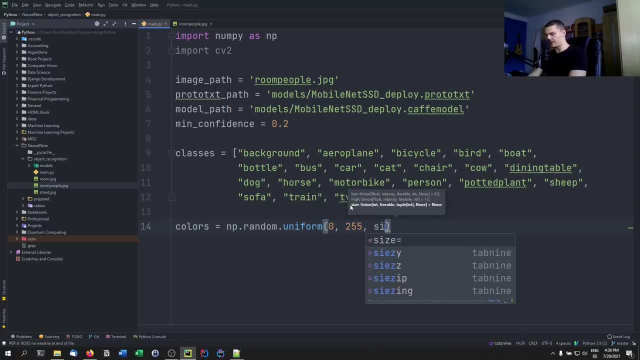 and the size that we're going to generate is going to be the length of the classes list. so we're going to have a color for each class and we're going to generate three values for it, so basically from 0 to 255. the problem is that sometimes this random uniform distribution will 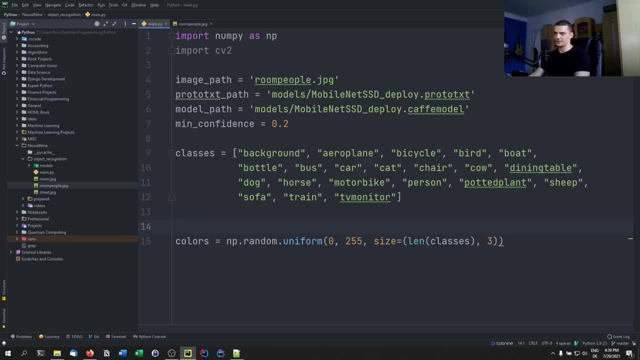 result in pretty bad choices for colors, so we're going to have very similar colors. if you want to use a seat, or if you want to always get the same results, you can use a seat. and in order to use a seat, you need to say nprandomseat. and by doing that, by specifying a certain value, here you're. 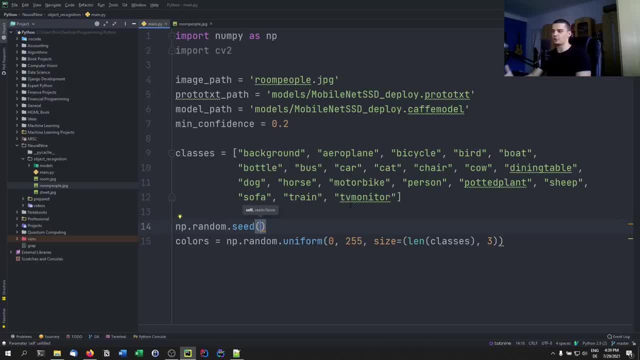 going to always get the same quote-unquote random result. it's going to be a determined random result and a seat that worked quite well for me is going to be the same random result. so we're going to use a seat that worked quite well for me is 543210. this worked quite well. got some good colors there. 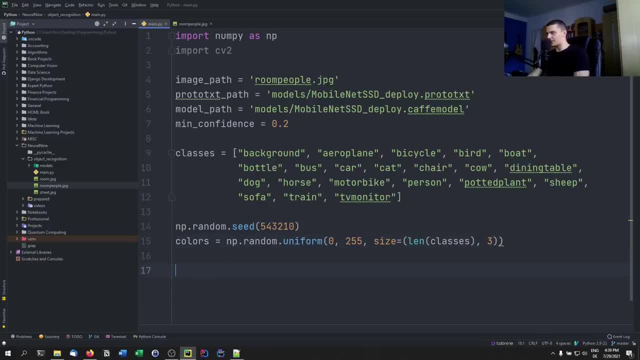 now what we're going to do is we're going to load the neural network into our script. we're going to load the pre-trained model. we don't need to train it, we don't need to do anything with it, we only need to load it, and then we need to feed some data into it for prediction. so we're going to say net. 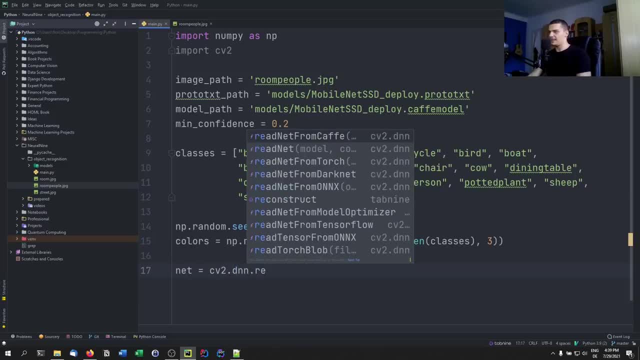 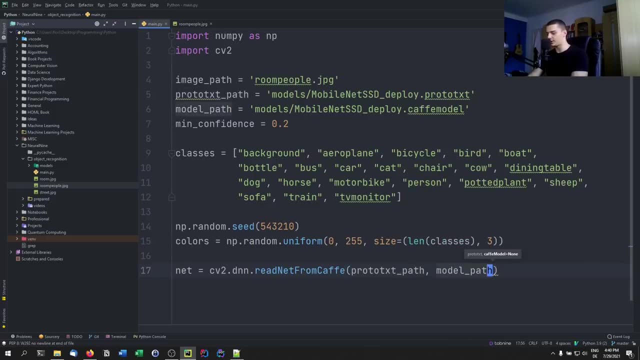 equals cv2.dnnread net from cafe. we're going to provide the proto txt path as the first parameter and the model path as the first parameter, and then we're going to load the neural network into our second parameter, and all we need to do now is we need to forward an image into that model and then 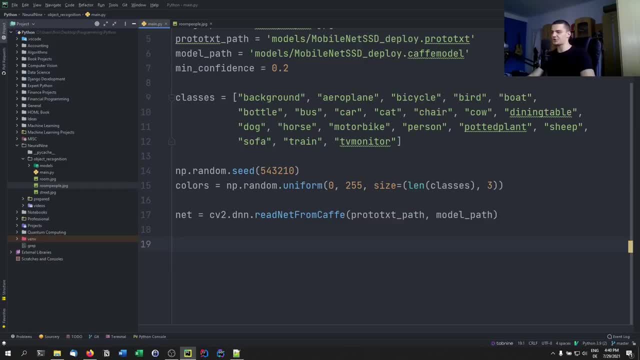 we're going to get the result of the detection or classification you could say, and we can then apply this and draw this onto the images. so what we need to do is we need to load an image, we need to resize this image so that it fits into the neural network, because the neural network accepts. 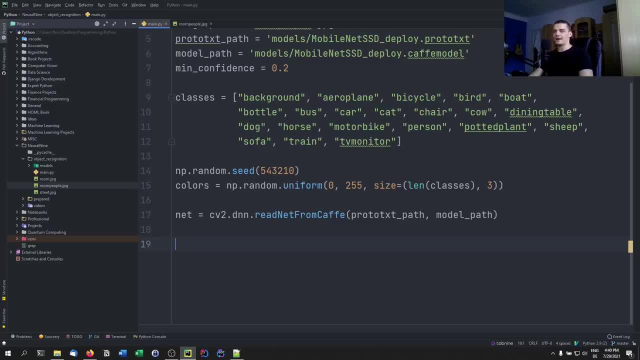 300 by 300 pixels, as far as i know, and then we need to get a prediction, then resize the image again and draw the detections onto the image. so we're going to first say image equals cv2.imread and we're going to read the image path here, and then we're going to save, we're going to store the. 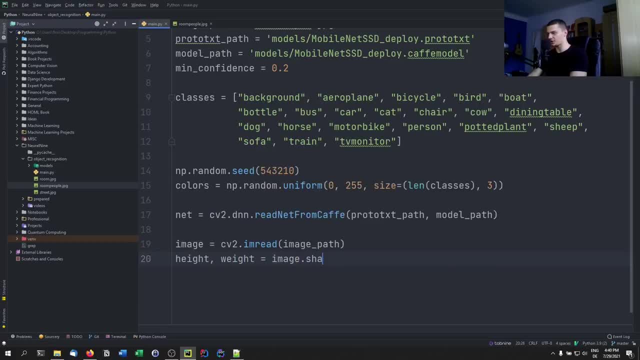 current shape. so we're going to say height and weight is going to be image dot shape zero and image dot dot shape one like that: uh, we're going to save it. and then we're going to create a blob object, a block object, uh, or a blob stands for 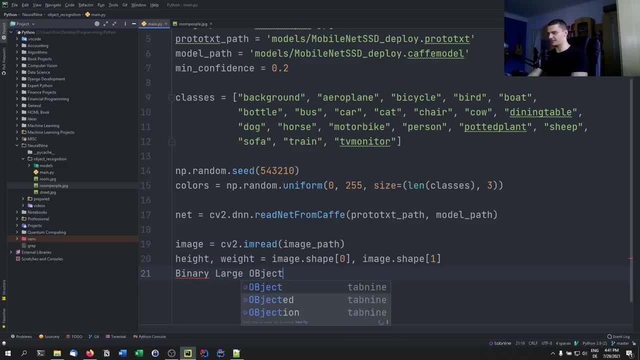 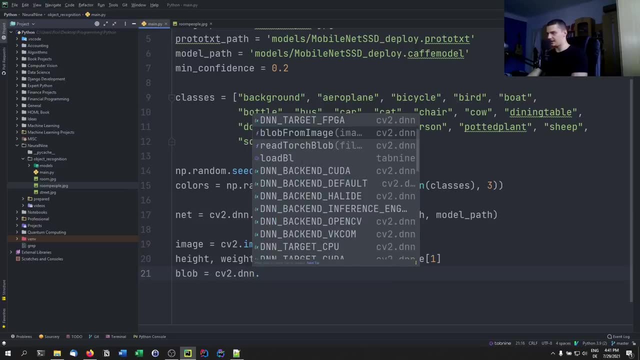 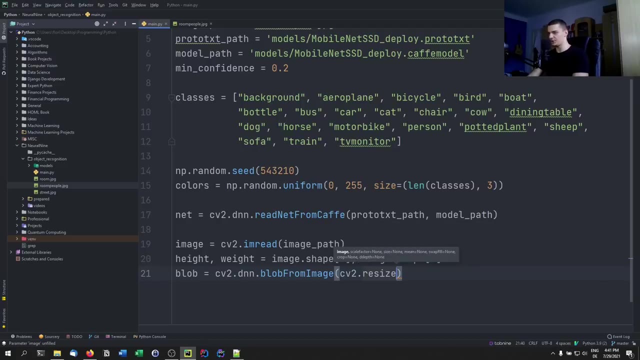 binary large object. this is what a blob stands for and we're going to say blob equals cv2.dnn. uh, blob from image, and we're going to say cv2.resize. so we're going to fit an image here and we're going to resize it to 300 times 300.. 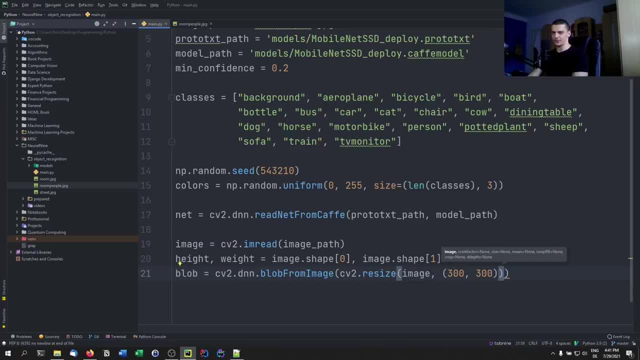 there you go. the second parameter is the scale factor. the scale factor, um, is something that you keep can play around with. uh, basically, what? the what's what the image is multiplied with? we're going to use 0.007 here, um, then we're going to specify the size of the image, which is obviously 300. 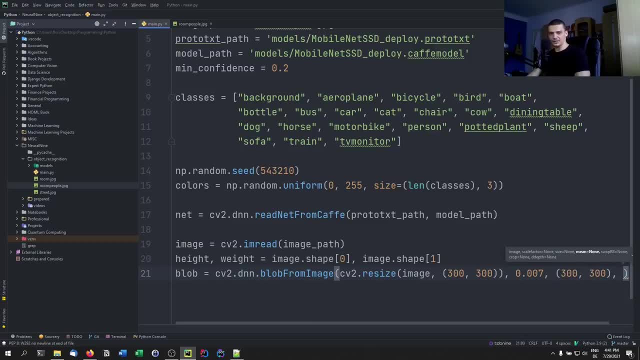 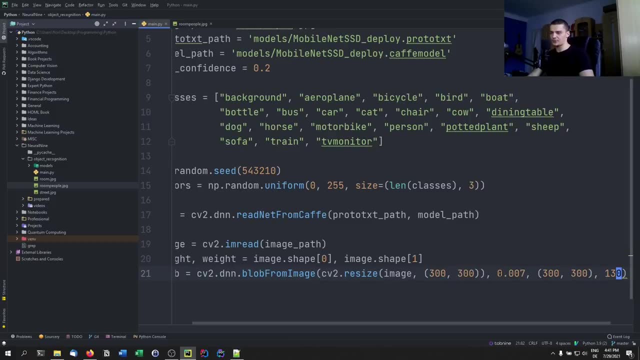 times 300 and then in the end, what was the last parameter? it's the mean, it's something that is subtracted. so in this case, 130, uh is a value. you can play around with these two values. with this value and with this value, you can play around and see if you get better results, if you. 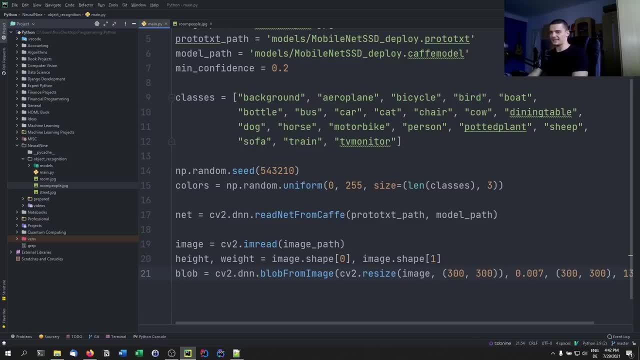 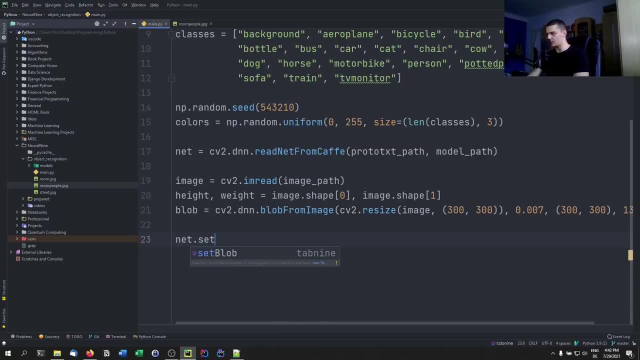 increase or decrease them slightly, just experiment around with that. but now we have this blob object and in order to get the prediction, what we do is we say net, dot, set input and we pass the blob object. so we have this blob object, we set it as the input of the net and now, as the next step, we say detected. 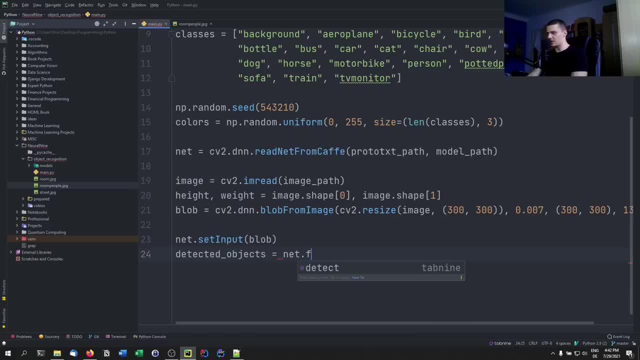 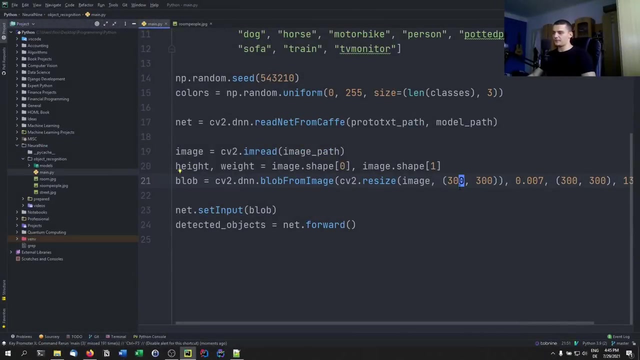 objects is going to be net dot feed- uh, not feed net dot forward. so we set the input, we forward, and then we get a result here as a return value. so technically speaking we're now done with the object detection. but of course we need to visualize it and as a first step we're going to just take a look at this thing here. that was 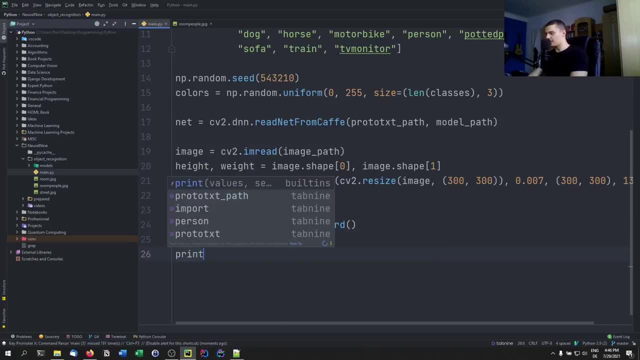 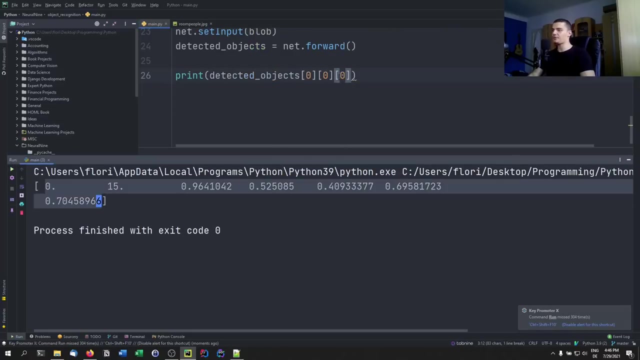 returned by the forward function, these detected objects, and we're just going to print detected objects and I'm going to say zero, zero, zero. I'm going to explain that in a second here. uh, when I run this here, I'm going to see that we have a bunch of values here, and how this works is that we have a bunch. 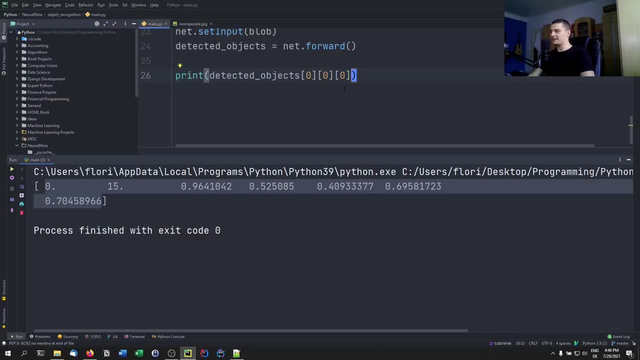 of different objects that were detected in the image, and this is the first object. this is the data for the first object that was detected in the image and if I want to change this to the second object that was detected, I just changed this third number here, so this now would be the second object. 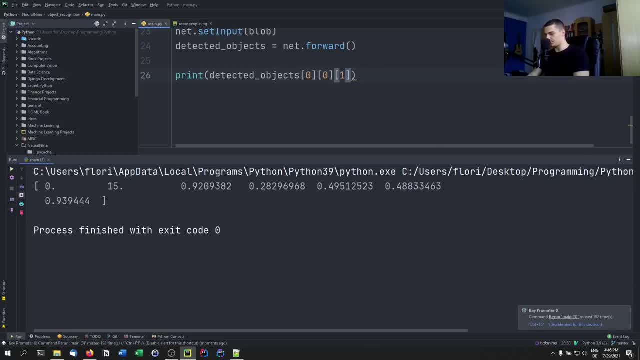 which was detected. as you can see here, I can change this to: provided we have enough objects, of course, I can change this to 15.. I'm not sure we have 15 objects. let's see. no, it doesn't seem like that. so let's say eight, the eighth, or actually. 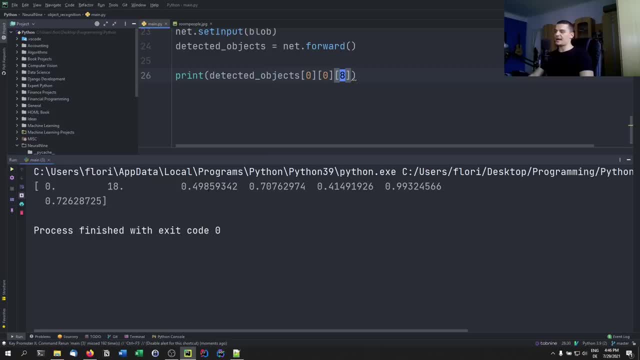 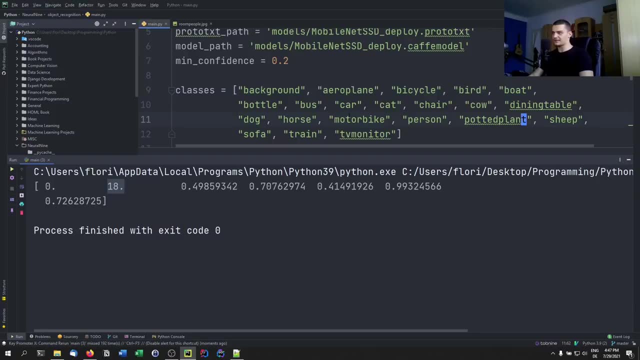 the ninth object was detected. you can see some other values and what we have here is this: thing is the class index. so 18 would be the 18th element of this list here, or maybe the 19th element, depending on how it's indexed. so this is the class. this is the actual thing that our model classified. 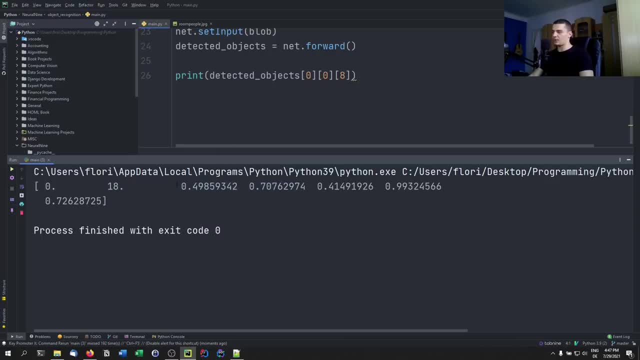 or detected, and here we have some coordinates. so, or actually, this here is the confidence and those are the coordinates. so this is the class, this is the confidence, this is the upper left X coordinate, this is the upper left Y coordinate and this is the lower right X coordinate and the lower right um Y coordinate, and how this works. is that all? 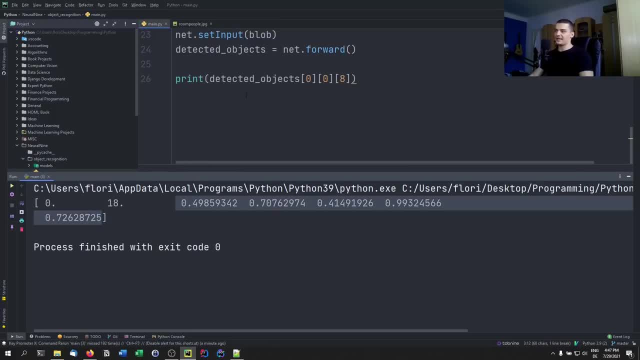 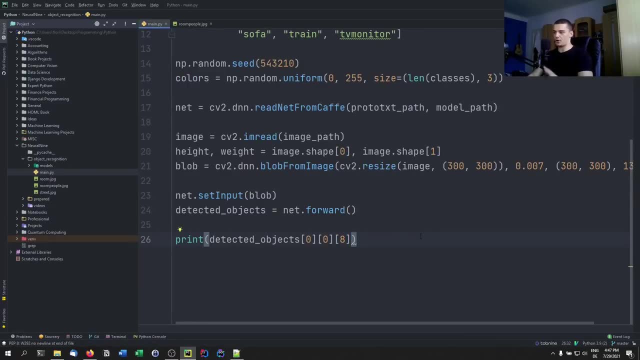 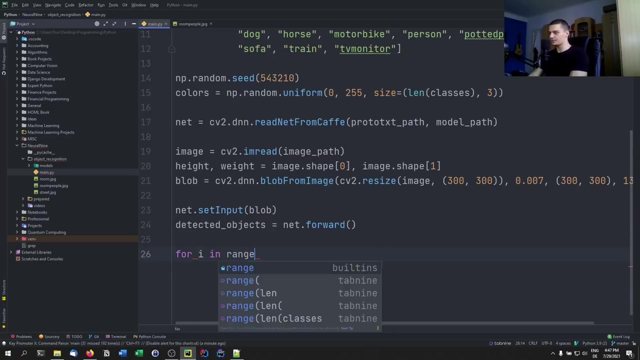 those values are normalized, so we can multiply them by the image height and by the image width and we're going to get the actual coordinates of these pixels. and this is how we're going to actually draw these rectangle, the objects. so let's get into coding. we're going to say for: i in range, and we're going to say for: 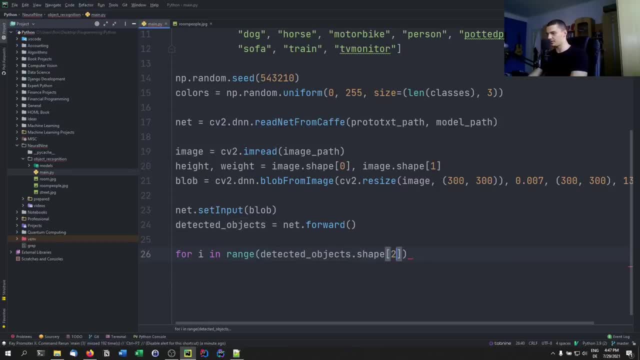 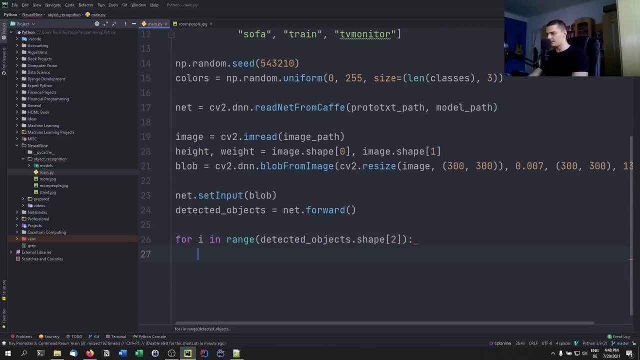 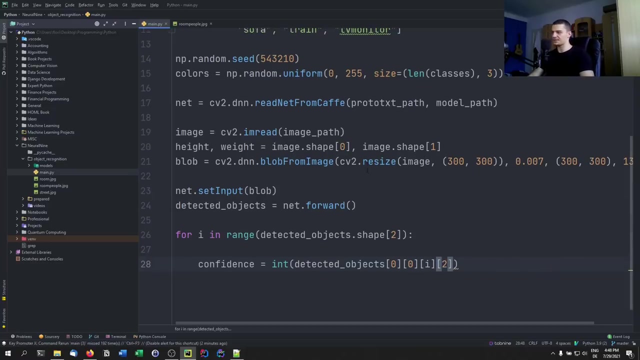 i in range detected objects. dot shape two. so depending on how many objects we have detected, we're going to say confidence for this particular detection. confidence equals int of detected objects. now, zero, zero i one. this is how we get the confidence. um no, this is the class index. sorry, this is two. is the confidence? one is the class index. uh, so we? 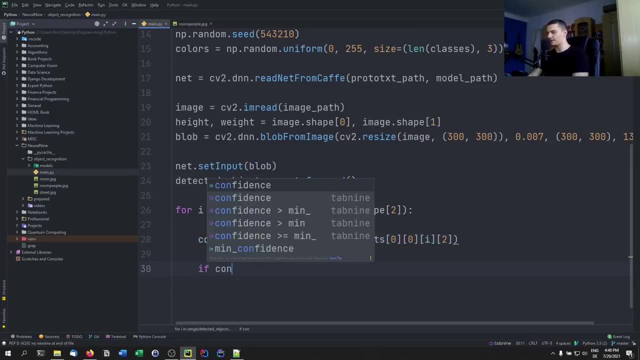 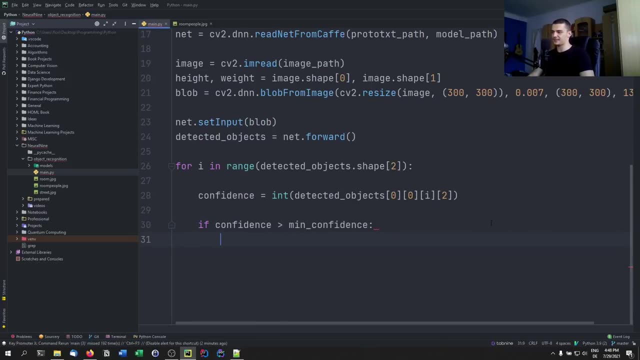 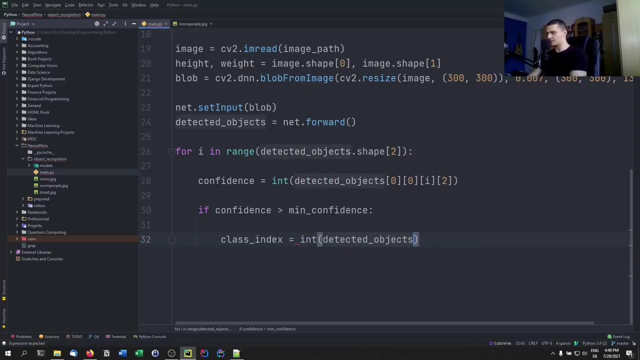 get the confidence like that, and what we do then is we say, okay, if the confidence is larger than the minimum confidence we need for detection, then we're going to draw a rectangle and put a text there. so we're going to say, okay, the class index that was recognized here is going to be int- detected objects, and i think we can. 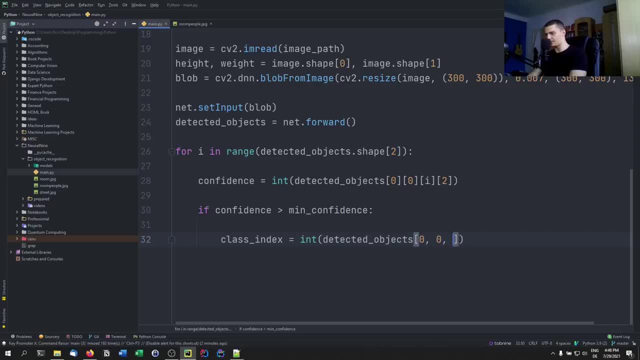 actually also specify like that: so zero, comma, zero, i one. i think this should work as well. so this, basically, is the same as this. of course, here we have a two and here we have a one, but i think the way of writing it is also fine, like that: um so, class index. is that then we're going to get? 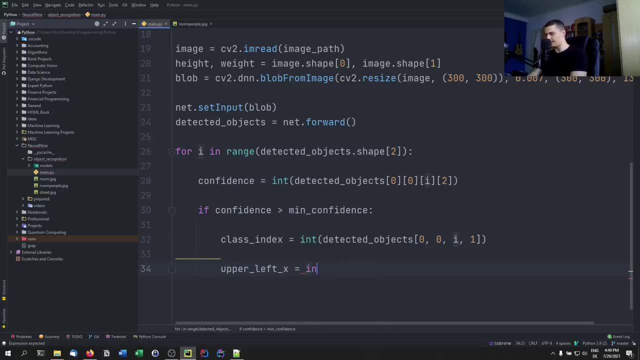 the coordinates. we're going to say upper left, x is going to be int, detected objects um, and we're going to say zero, zero, i, three important. we need to multiply this with the width because of course we have this normalized value for x and we want to multiply it with what? 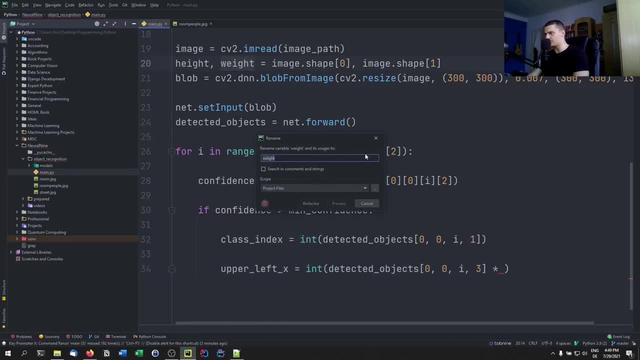 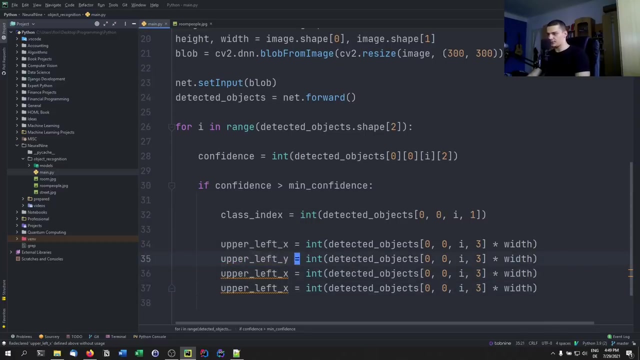 we had uh here. oh, by the way, i see that i used uh weight here. we want to have this as width, obviously, um, and we're going to multiply that by that value. so we're going to copy that and we're going to say: upper left y is going to be index four times height, like that. and then we're going. 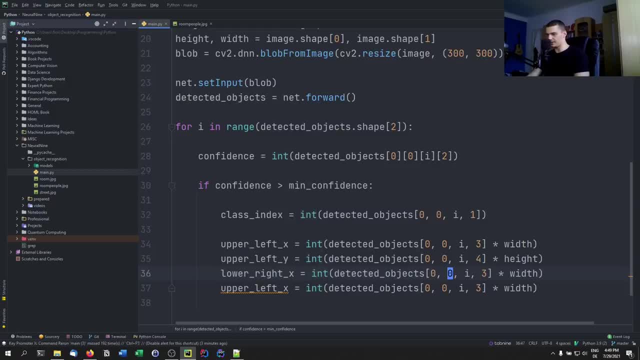 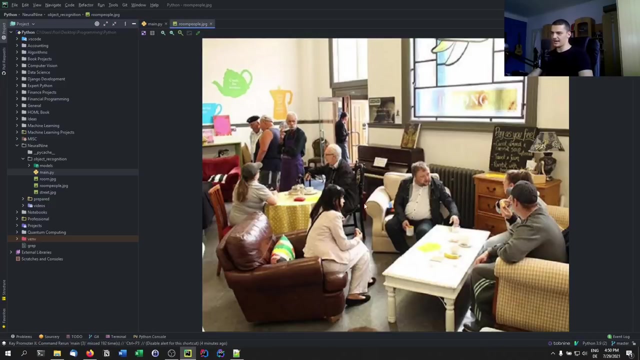 to say, lower right x is going to be five times width and then lower right y is going to be six times height. so we then have the exact coordinates of the corners, and you need to think about it like that: if this is the upper left and this is the lower right. i know. 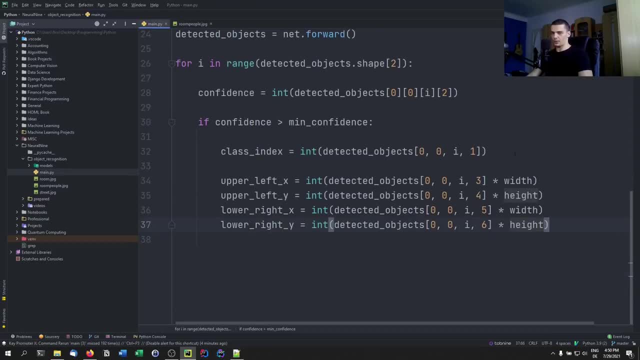 that all this is the person. uh, this is how we're going to plot this um, but first we're going to craft a prediction text. so we're going to say prediction text is going to be an f string and we're just going to say classes, class index. so yeah, actually this is um if we have the index 18. 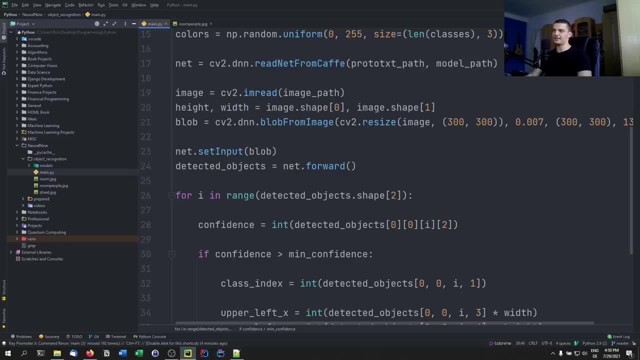 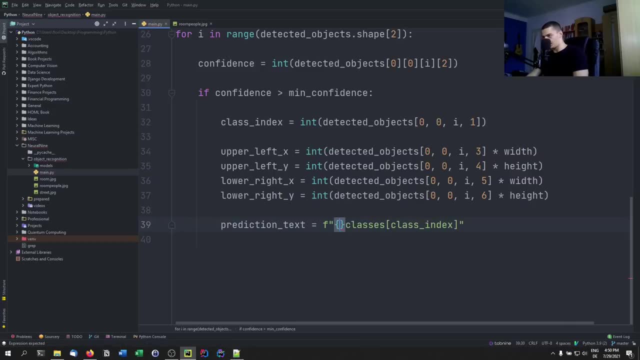 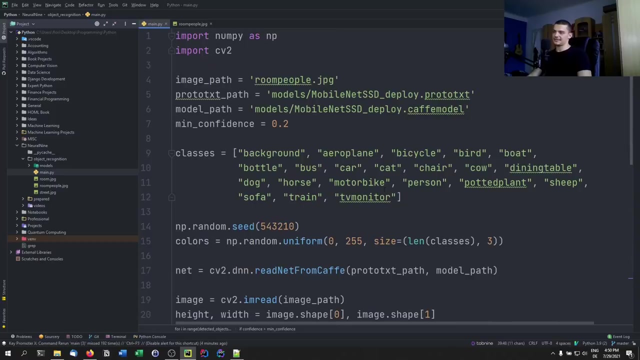 this means that this is the class 19, so the 19th class, but it's the index 18 and we start at zero. so, uh, that was what i wanted to say before, and we start here with the class index, uh, the class of the class index. so if we have 18, it's going to go to index 18 and 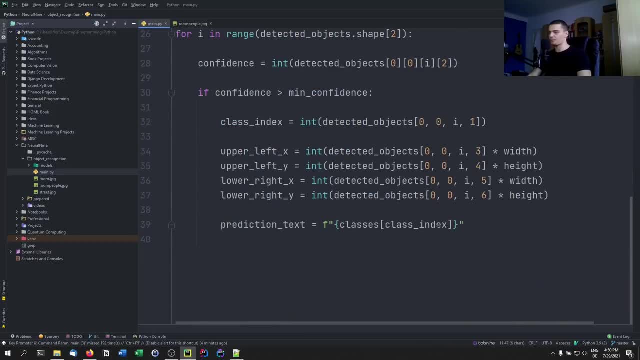 give us that, uh, give us that string here, and we're going to have that in the text. and as a second thing, we also want to know the confidence. how sure are you that this is whatever it is or whatever you think it is? so we're going to say confidence, we're going to format that as: 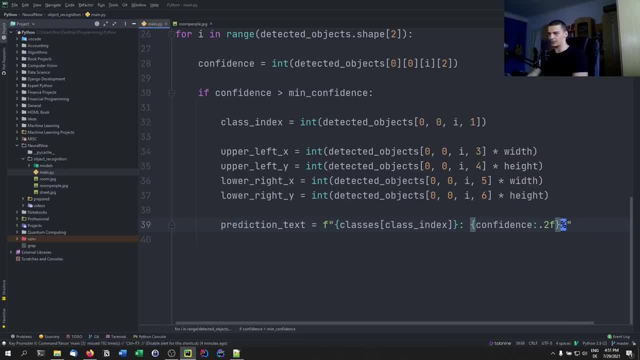 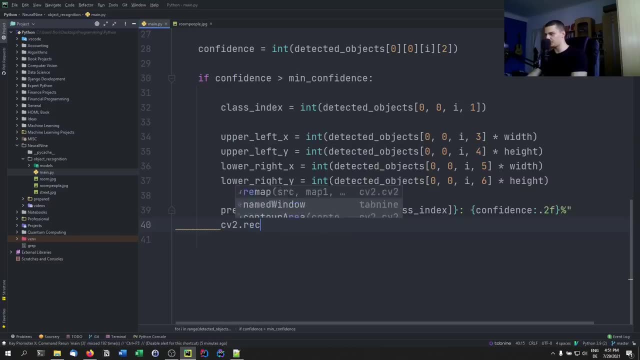 uh, two decimal places, a float with two decimal places. so we have the prediction text and we now only need to draw a direct angle and put the text there. so we're going to say cv2 dot rect angle, and what we pass here is, of course, the image itself, then a tuple of upper, left, x and upper. 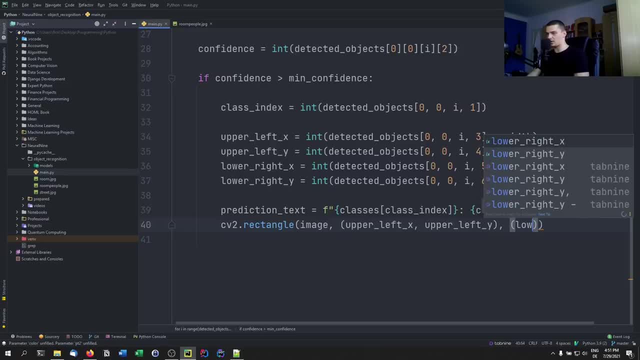 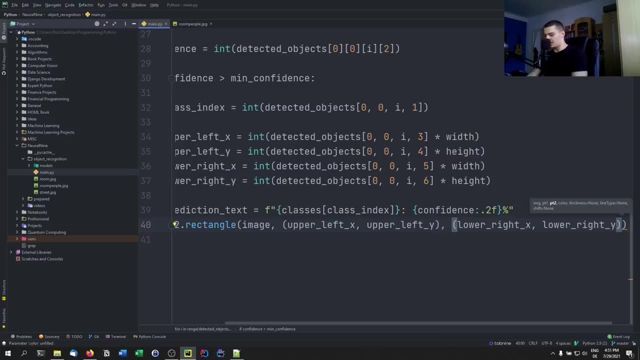 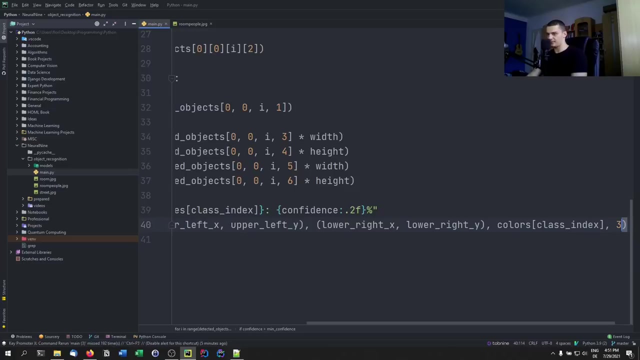 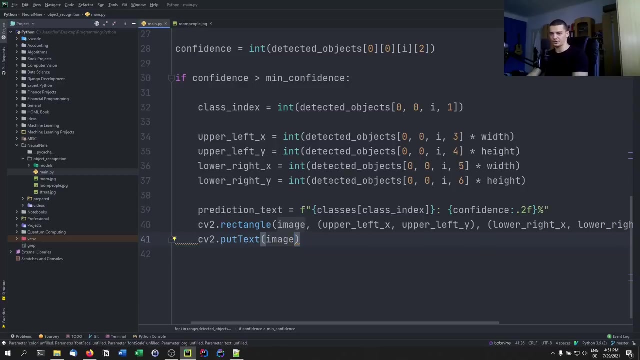 left, y, as a second thing, the lower right x and the lower right i, uh, y, not i, and then of course the color that we have. so colors, class index, hopefully well randomized, and then three, uh, and finally we say cv2 put text, and i have a bunch of parameters here, i just need to. 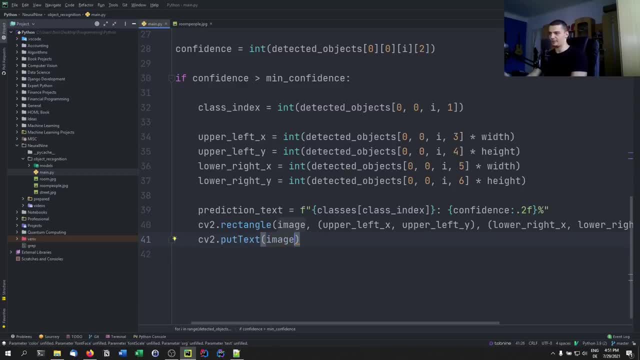 look at them, because parameters are always confusing me. never learn parameters, uh. never memorize parameters. always look up the documentations or your sample code, uh. so here we have image again. we have prediction text that we just crafted, and then we have the position. so we're going to say upper left x, and then we're going to say upper. 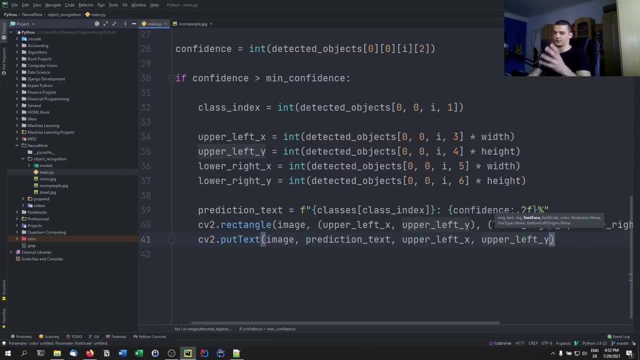 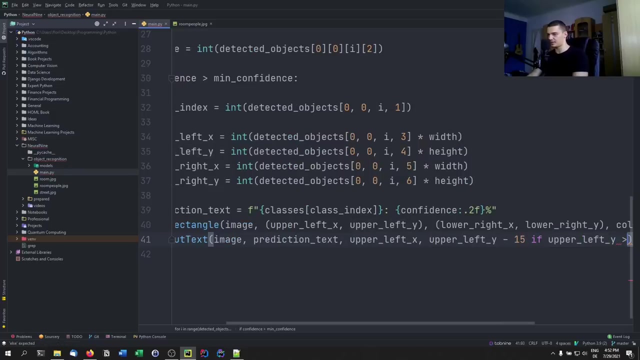 left y minus 15. if this is for the text, if the text fits in, we're just going to put it there. otherwise we're going to put it either above or below. so we're going to say upper left y minus 15 if upper left y itself has enough space to put that there. so if it's above 30, else we're just. 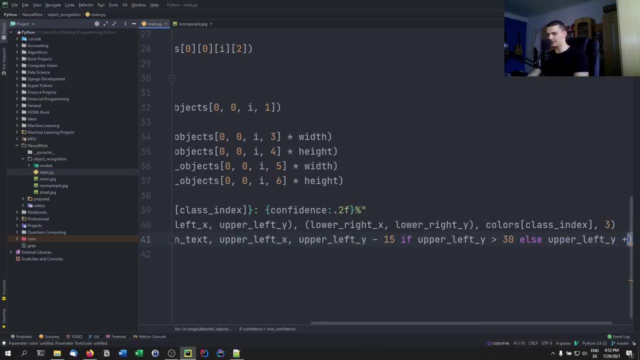 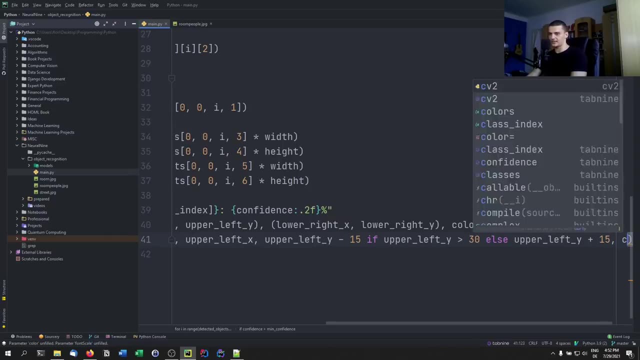 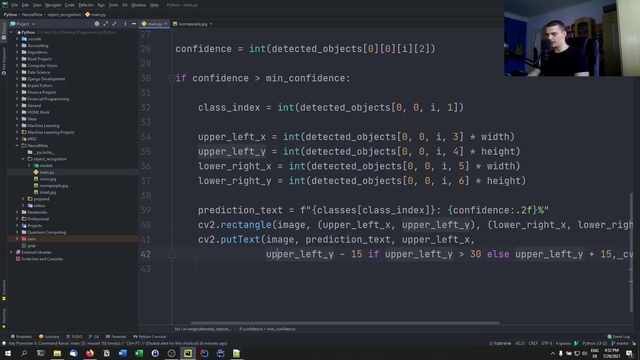 going to say upper left y plus 15.. right, so like that. and then we're going to also pass the font so cv2. maybe we should do a line break in here somewhere. let's just see, there you go and let's make one more cv2 dot font. 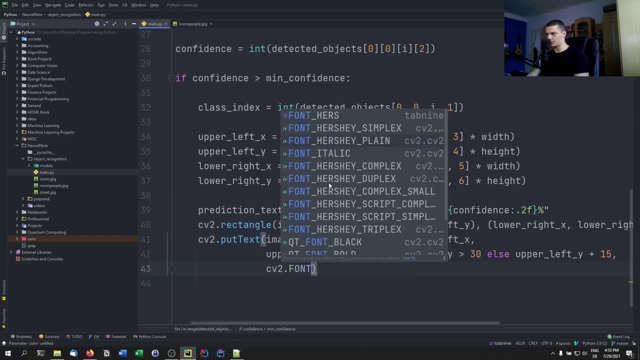 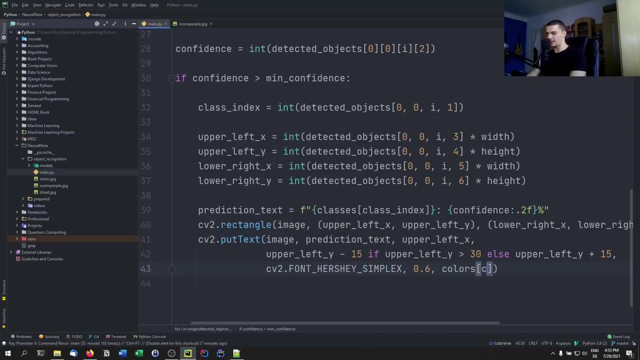 come on font and we're going to use the simplex. where is it this simplex font here? 0.6 here and then a color, again class, index and 2.. by the way, all those parameters are just designed so they're not not important for the actual detection process. you can play around with them, you can change them. 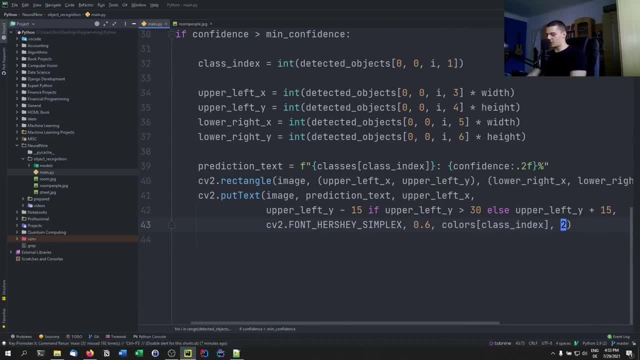 this is just design stuff and once we have that, we're done and we only need to show the image. so we're going to say cv2.im- show some title, i don't know some detected objects or something, and then the image and cv2- dot weight key zero. and maybe we should also say cv2- destroy all windows. 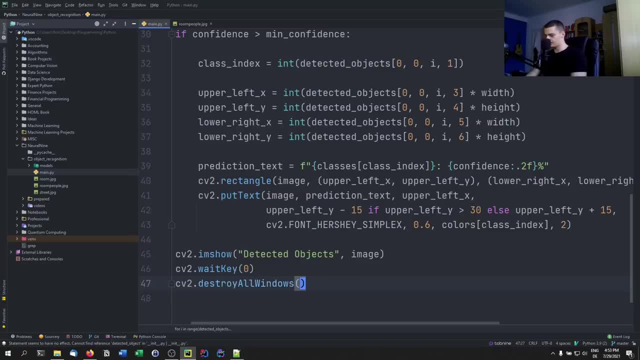 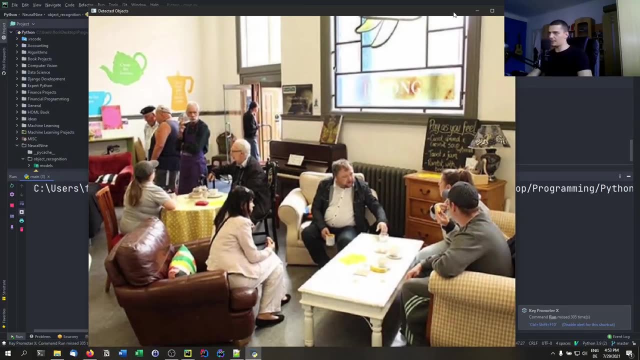 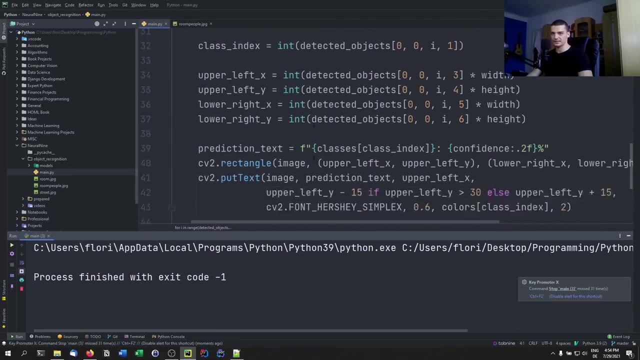 there you go. so let's see if we didn't make any mistakes and if it works, there you go. uh, but we don't have any predictions. why is that? did we have? did we forget something? some scaling or something like that? let me just see. um, maybe let's turn down the confidence, maybe that's the. 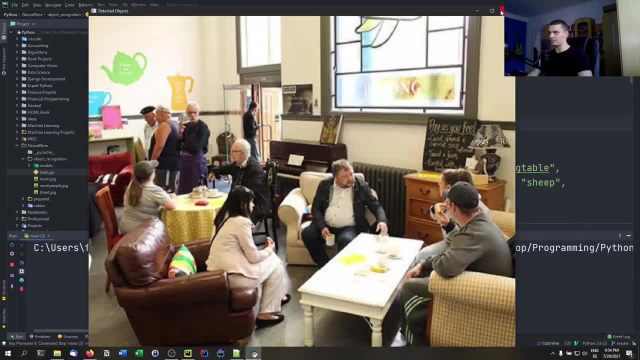 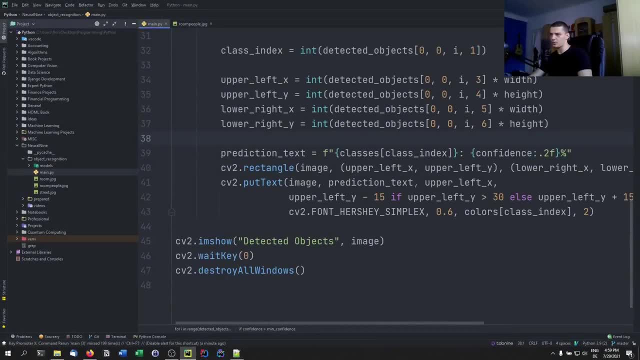 issue, but i don't think so. i think we have some other problem here. okay, i'm going to take a look at that and then come back to you. all, right, it wasn't too much of a big deal. uh, we have two problems. first of all, we have to pass a tuple here, so in a put text function when we pass upper left. 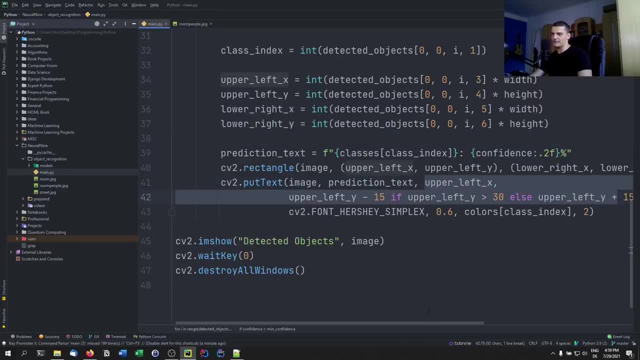 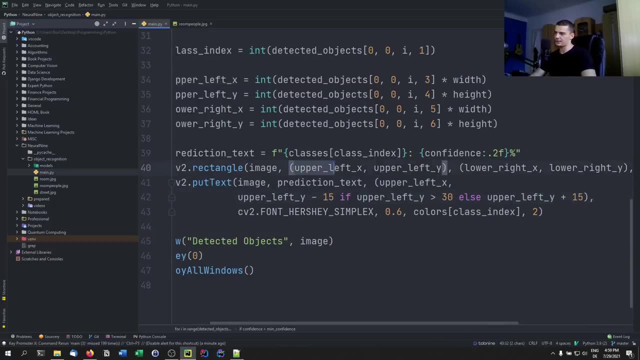 x and this uh statement here with the if and else. we need to put that into a tuple. so we need to start here and end here. so we need to start here and end here. so we need to start here and end here, it here, because the same way that we put it here in a tuple, we need to put it here in a tuple. 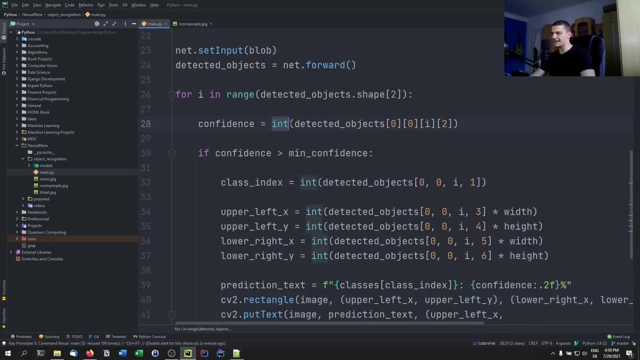 and, second of all, we have the problem that we're using in here even though we shouldn't be using in here, because, for the confidence of course, we're never going to get anything um other than zero point something. so we're always going to get zero if we go within. so that was not a very 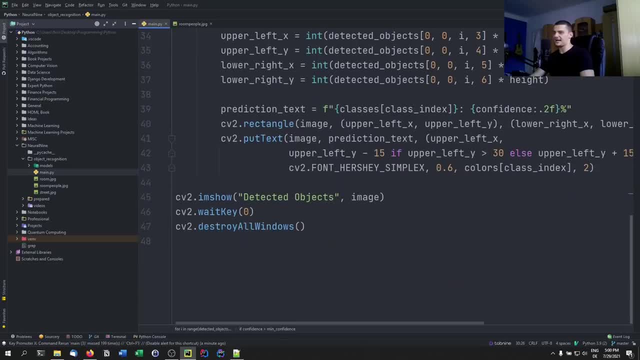 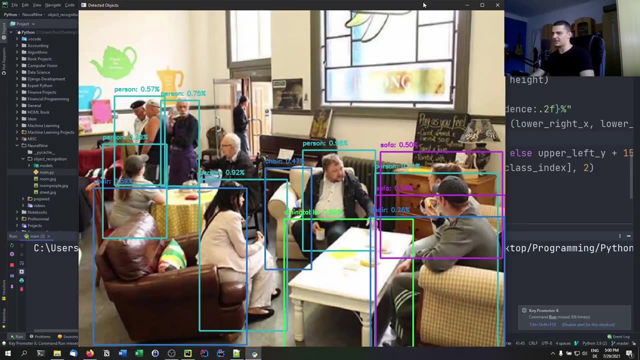 intelligent choice. we need to remove this in here. this was a mistake and we need to put this into a tuple and then it works, because then i can just go with run main and you can see that we get the classifications here. you can see 50 that this is a sofa. this is not quite right. uh, it says this is: 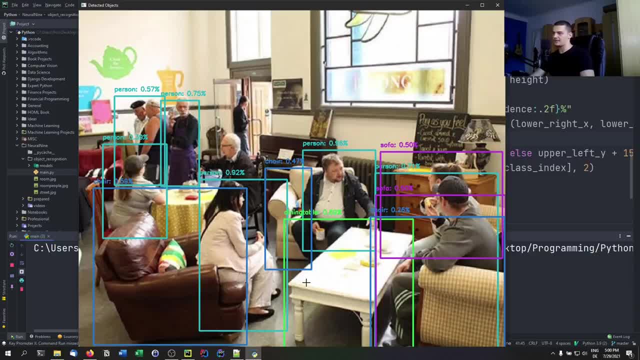 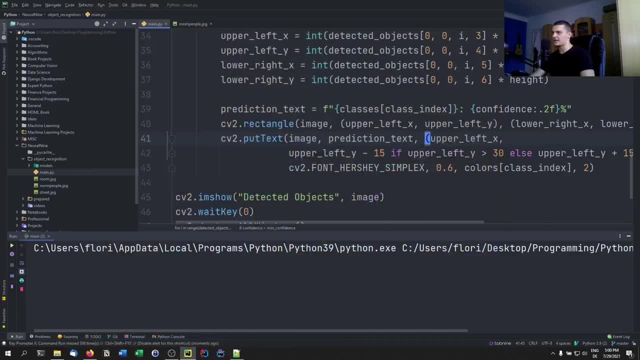 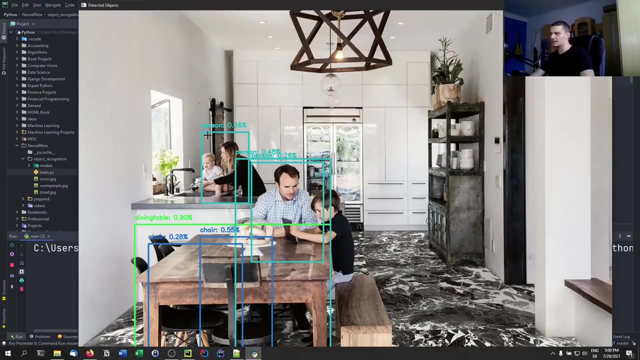 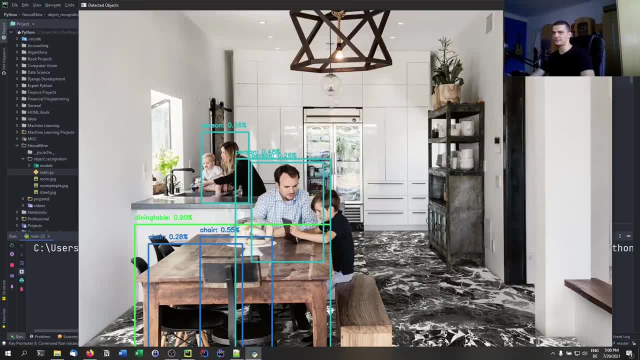 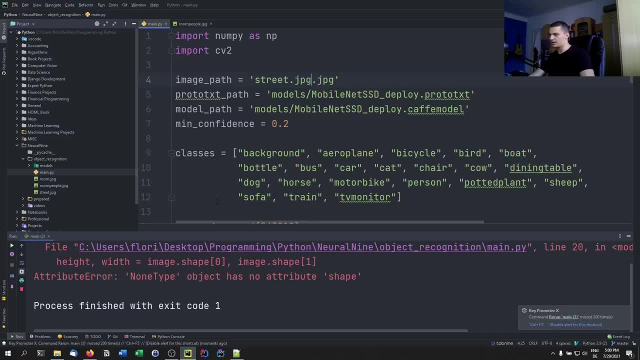 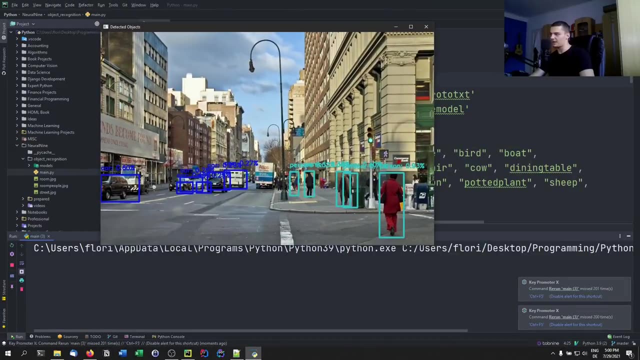 person, person, dining table, chair and chair. so this is fine, now let's go to the street and we're going to see that, uh, what is it? oh, jpegjpeg, no, just streetjpeg. and then you can see: okay, we have car, car, car, car, car, person, person, person, person, person. 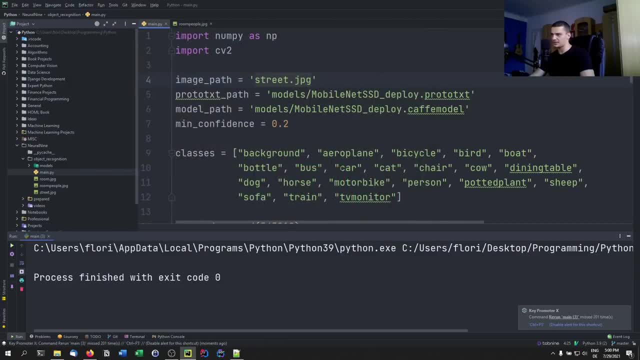 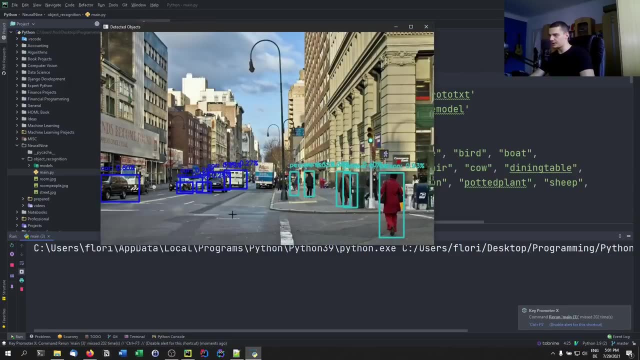 uh, now i don't know if we have something like truck. doesn't seem like we have something like truck, maybe bus, but it didn't recognize a bus because there is no bus. uh, do we have any bicycles here? no, i don't see any. so this is quite, uh, quite good. as you can see again, if you change the seat, you're. 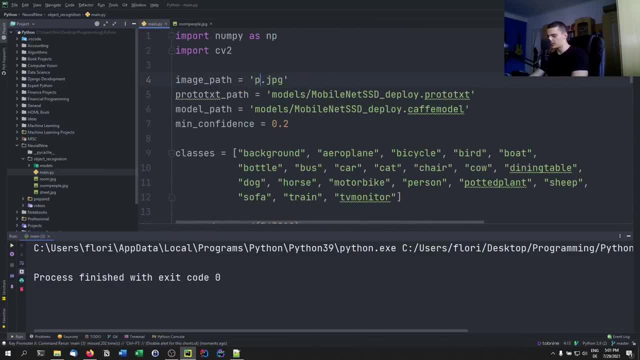 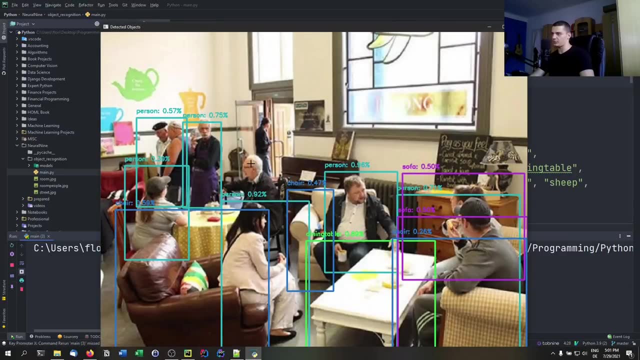 going to get different colors. so let's compare again the first image that we have. what was it? room, people dot jpeg. and let's look at the colors. you can see that we have turquoise for person, we have blue for chair, we have green for dining table and pink or purple for sofa. if i change, 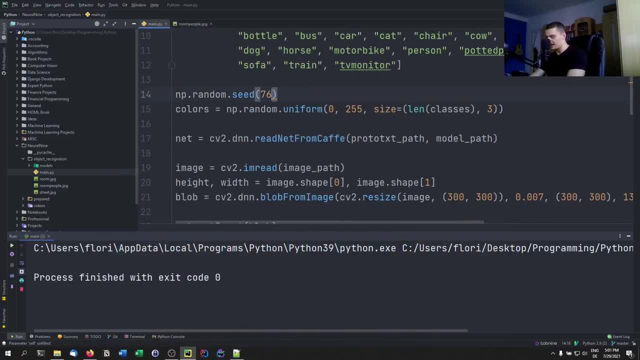 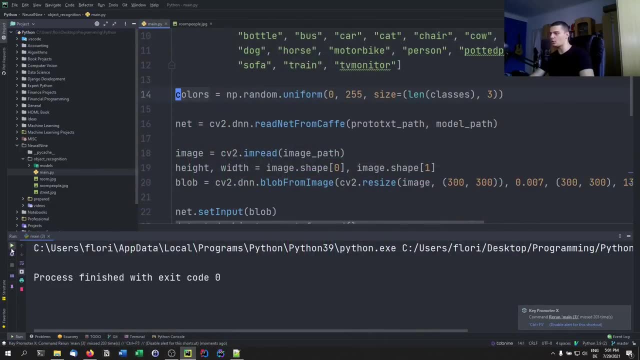 the seat, we're going to get different um values. so if i do something like that, we're going to get different colors, as you can see, and if i don't provide any seat at all, we're always going to get different colors. so one time we're going to get it like that. another time, if i run this, we're going to. 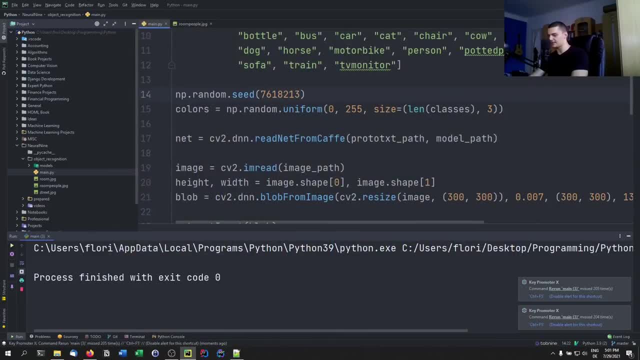 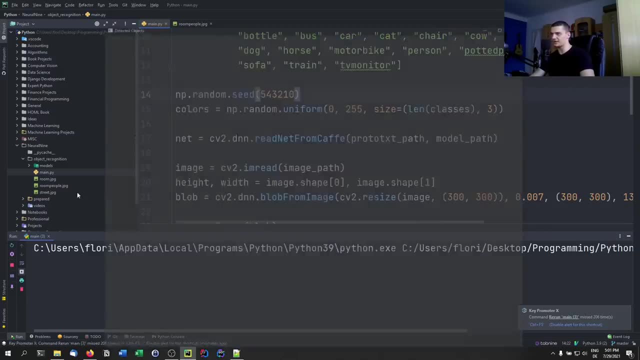 get a different color. so if you want to keep it consistent, you provide a seat. five, four, uh, what was it? five, four, three, two, one, zero is a pretty good one, in my opinion. you're always getting, uh, getting the same colors as you can see here, and this is how you implement object. 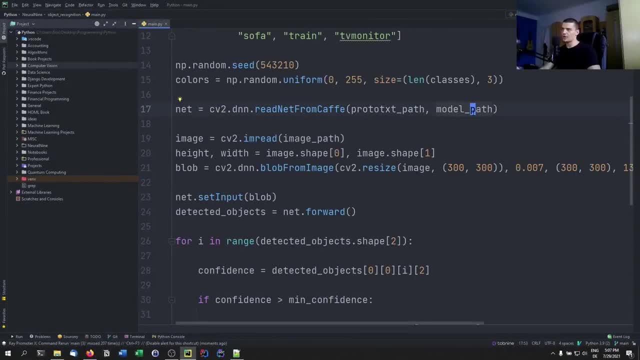 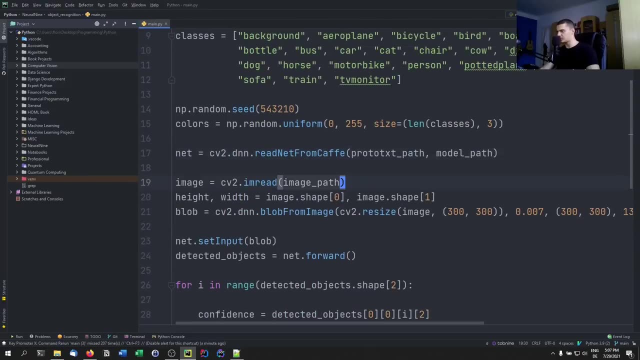 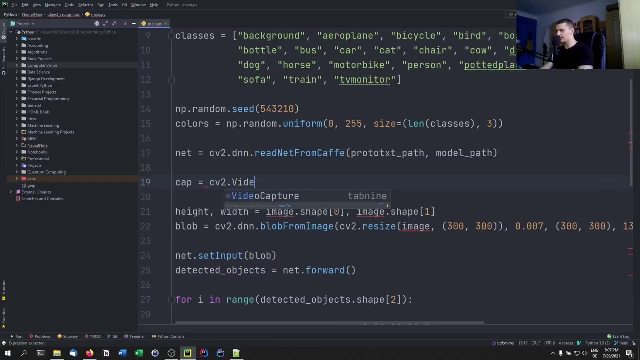 detection in python. now, last but not least, i also want to show you how you can apply that live to your camera data. so let's go ahead and uh, not load a static image like this one. let's get rid of that, uh, and let's make a camera here. let's say: cap equals cv2, dot video capture, and we're going to. 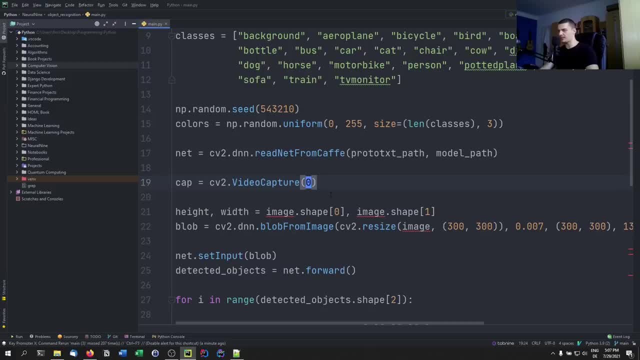 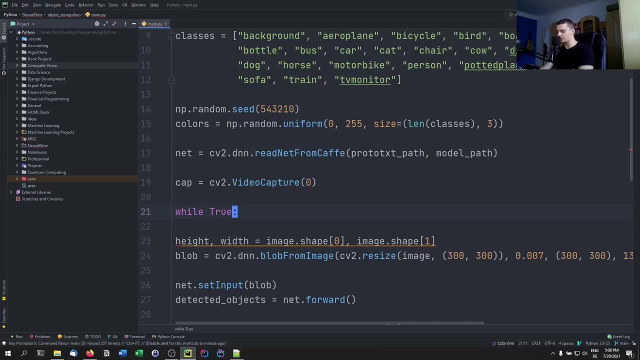 pass zero, which is the first camera. i only have one, so it's going to pick this one anyways. and then we're going to say, while true, and what we want to do all the time is we want to get a red and frame, or actually, let's call it image. 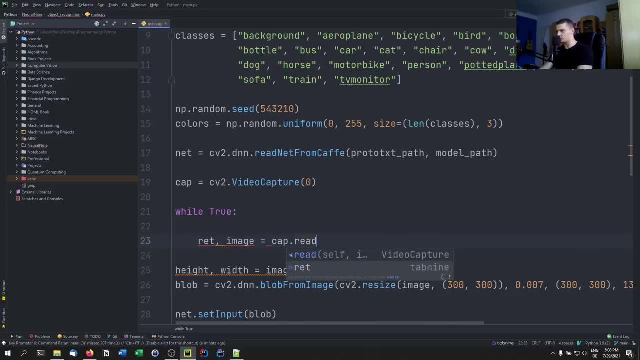 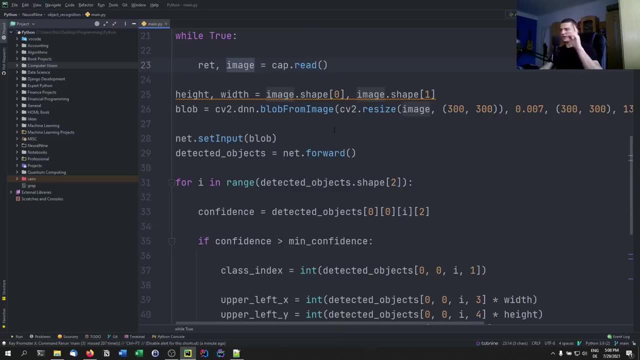 red and image from cap dot read. so we're going to constantly read the camera data and, as a result, we're going to get the image from the camera. so, this image that you see on the top right corner at the moment, it's going to be the image that we feed into the neural network, so we're going to 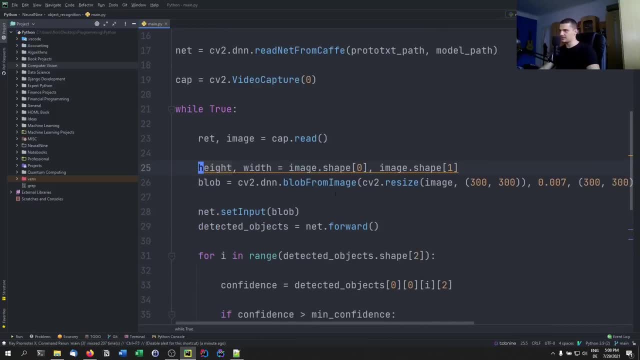 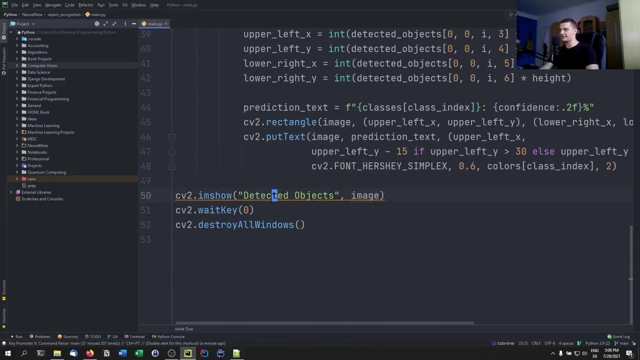 take all this and indent it, and then the process is the same. so we get this image here. this is the second parameter. actually, we can name this to just be underscore, because we're not going to use it. we're going to name this image, we do the same process that we did before and then we classify. 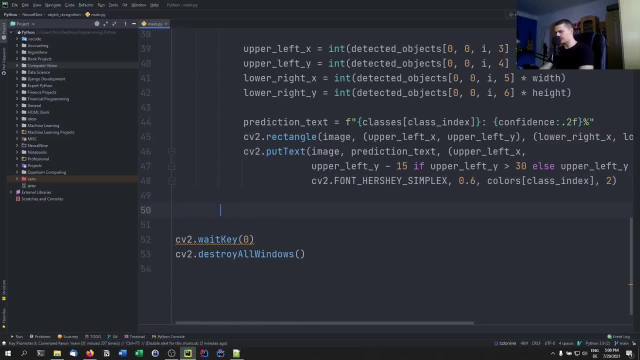 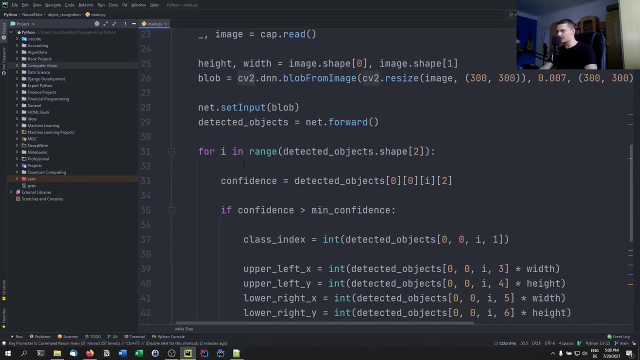 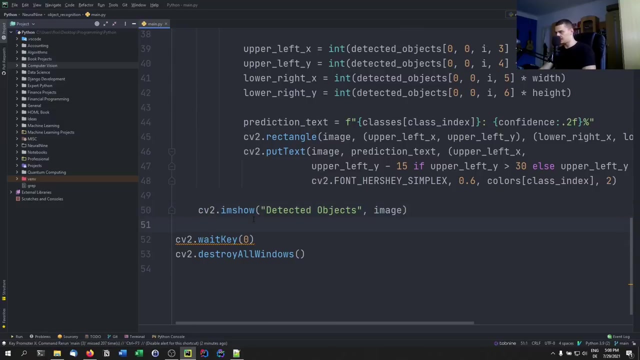 everything, and this im show here needs to be um inside here as well. so we're going to just um and then this here as well. let me just see if it's correct. every time, yeah, with each iteration, we're just going to show the image, and i think that should actually be it. uh, we're just going. 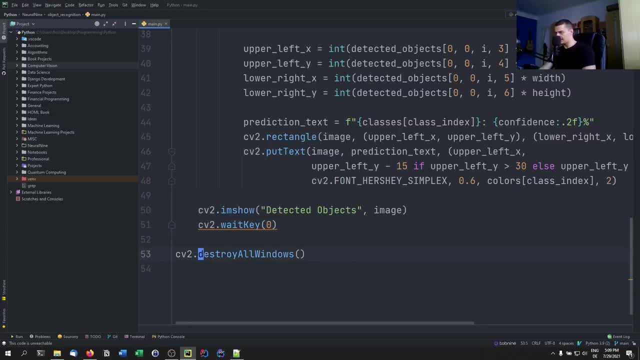 to put the weight key in here as well, and in the end, we're going to do destroy all the images. so we're going to say that this is the image that we want to show to the camera. so i'm going to go ahead and just remove this image, and then we're going to do a demonstration. 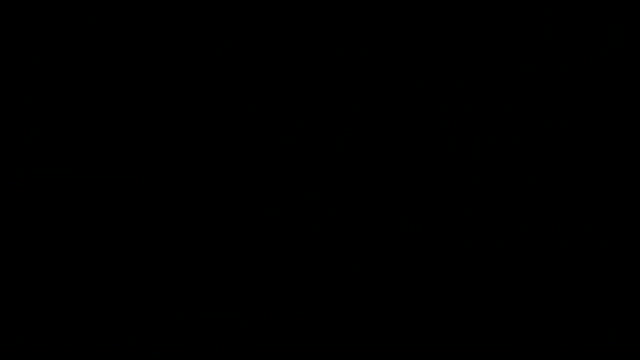 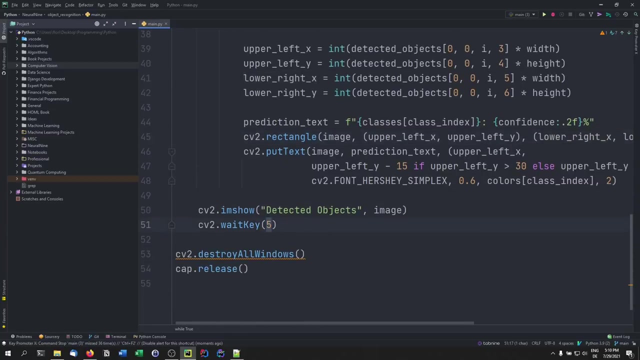 so i'm going to go ahead and just remove this image and then we're going to do a demonstration, all right, so i have now disabled the camera for recording and we can use it in python. one thing that i changed here is i changed this from zero to five. this is important because zero. 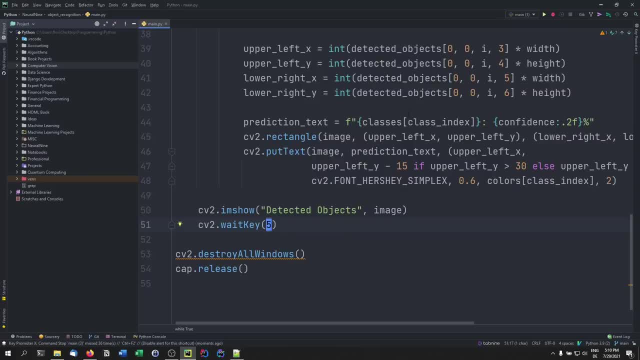 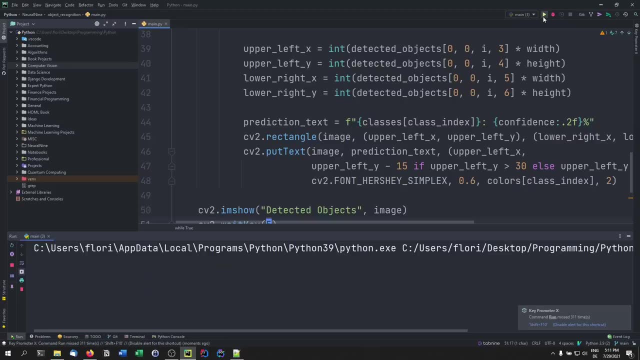 will just freeze your image. you want to have it at one, two, three, four, five, i don't know what. uh, just pick a number here. this determines the fps. uh, just don't pick zero, and then you're going to pick zero and once you have that, you can just run this and you're going to see that it's going to. 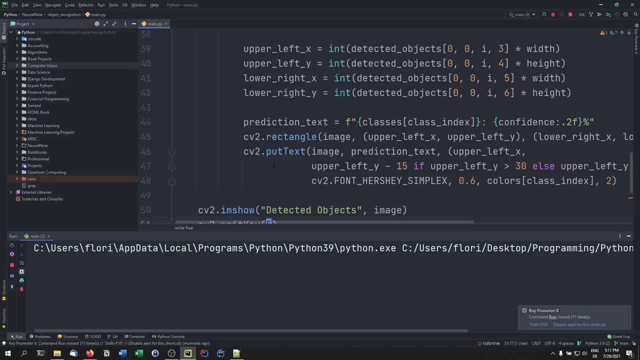 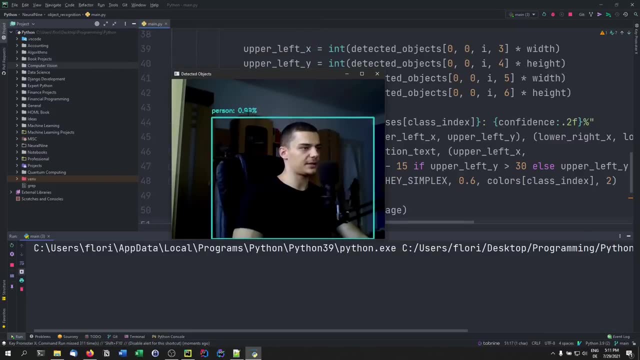 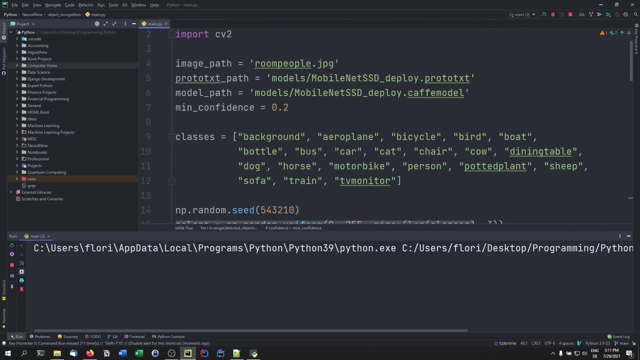 use the camera data for the object detection, um, and once it's loaded, you should see a camera. there you go um, so you can see here person with 99 confidence chair. now, this is not a chair. back then. uh, back there. uh. the problem is, of course, if we look at the classes here, there is not really much. 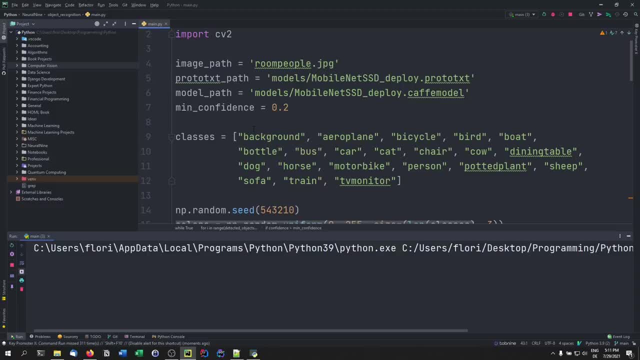 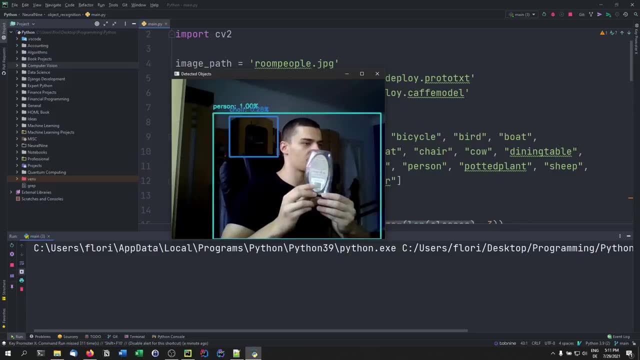 that it can classify maybe a bottle. do i have a ball in here somewhere? not really, i have honey. let's see if that works. so, yeah, i mean, yeah, it classifies it as as a bottle, as you can see here. i mean it's not a bottle, so we cannot really blame it for not classifying it as a bottle. uh, but it seems to. 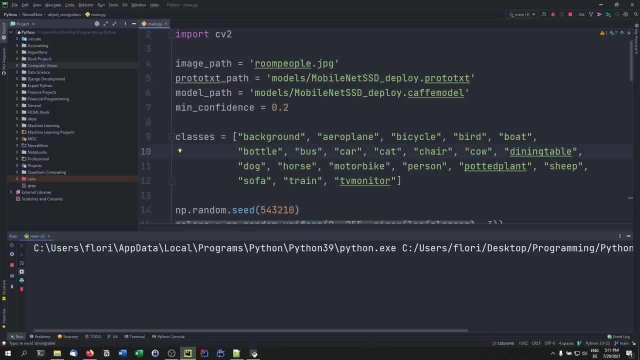 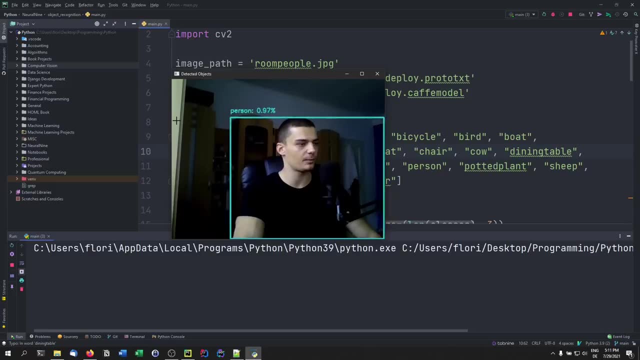 work kind of: uh, we can classify sheeps and horses. i don't have sheeps, horses, dogs here. uh, the chair, i don't know. maybe if i stand up it's going to classify this as a chair, or maybe if i turn around a little bit here, no, however, as you can see, it works live with camera data as well. all. 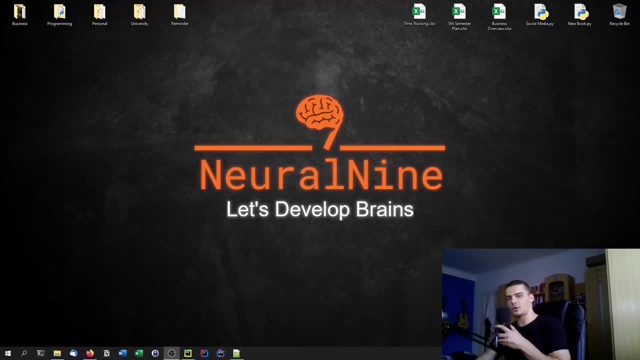 right. so that's it for today's video. i hope you enjoyed it. i'll see you in the next one. bye, bye. you'll learn something? if so, let me know by hitting the like button and leaving a comment in the comment section down below. and, of course, don't forget to subscribe to this channel and hit. 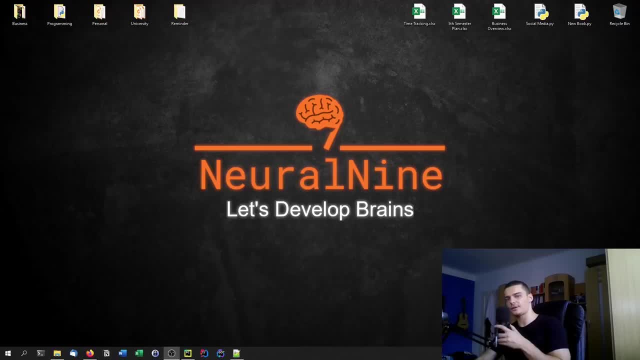 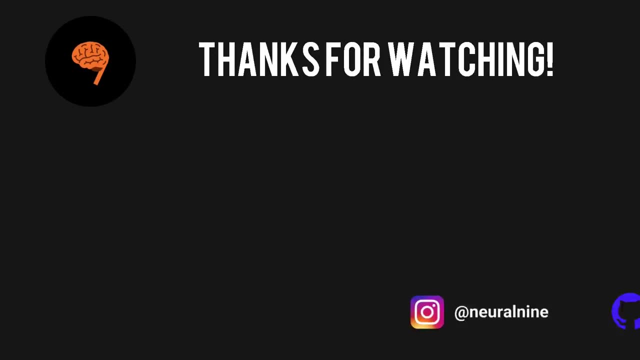 the notification bell to not miss a single future video for free other than that. thank you very much for watching. see you in the next video and bye. 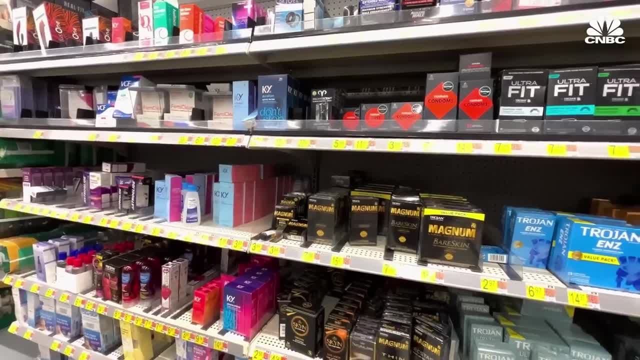 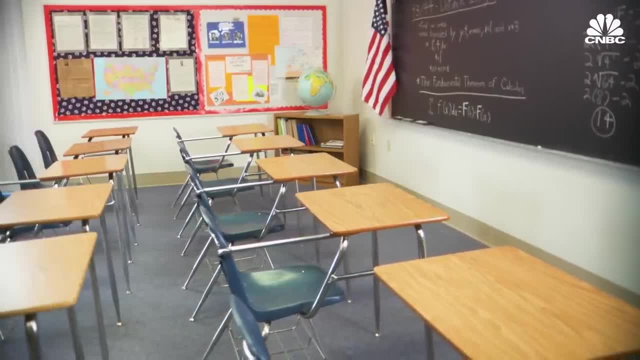 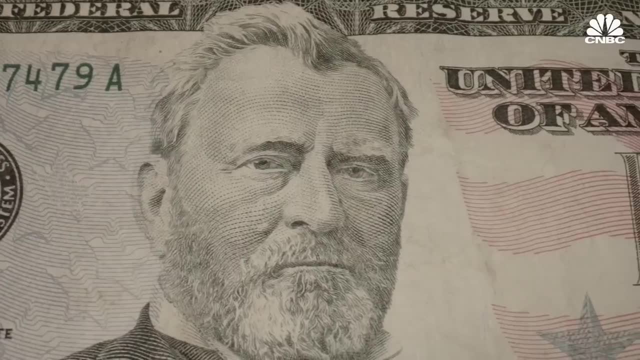 Sex education is an economic justice issue. We could have kids learn more in school if we raise standards. We understood our curriculum and we were basically thrown a curveball. I don't think the wages match sort of the level of expectation of the position. Teachers literally have the 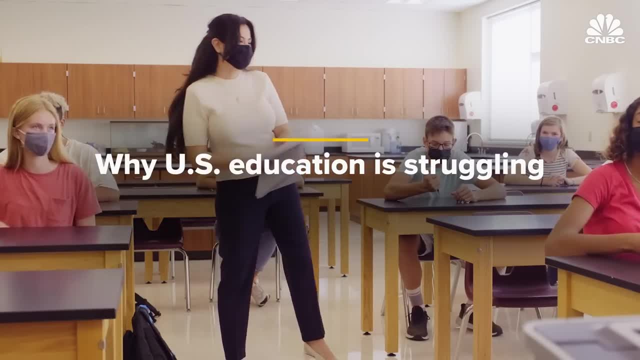 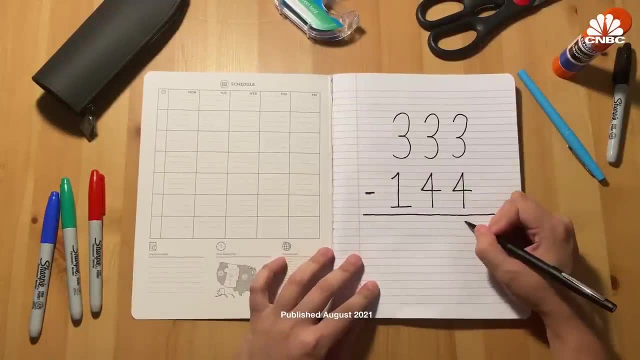 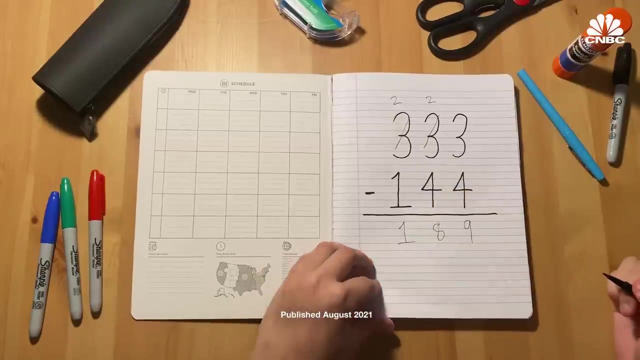 future of the country in front of them every day. How would you solve this equation? For most of us, it's as simple as following a series of familiar steps to get us to that answer. Now, remember this: This is how students under Common Core 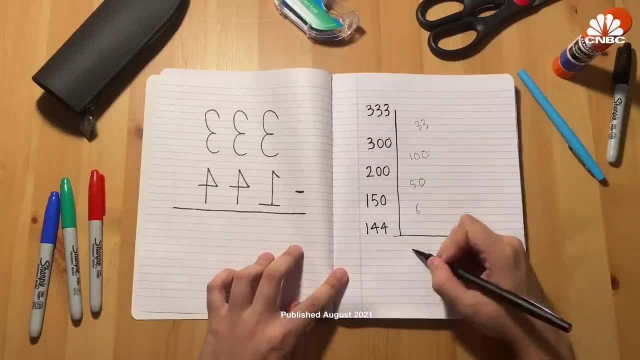 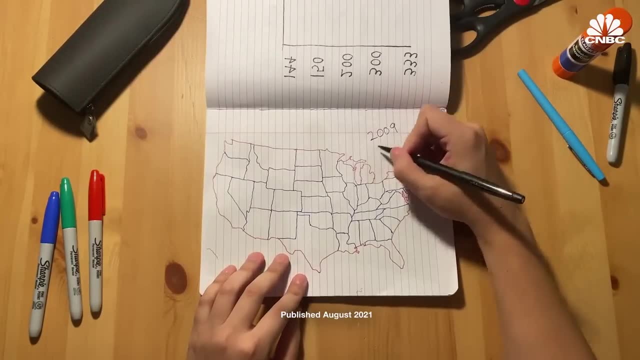 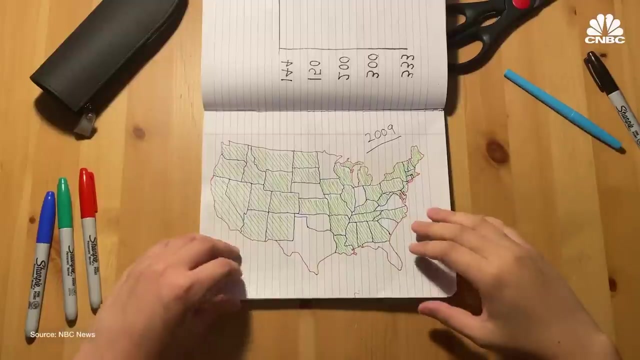 were taught to solve the exact same question. First adopted in 2009,, Common Core was an ambitious initiative to revolutionize the American education system. 41 states, the District of Columbia and four territories- National leaders, from Bill Gates to President Obama, supported the idea of the Common Curriculum and it. cost an estimated $15.8 billion to implement. They thought standards were just too low in the US and that we could have kids learn more in school if we raise standards. Quite frankly, they didn't really trust the schools to do this on their own. 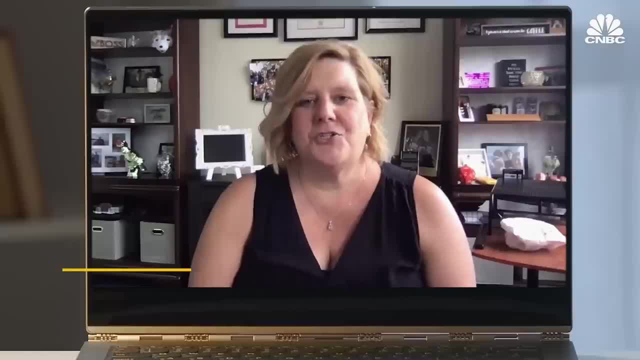 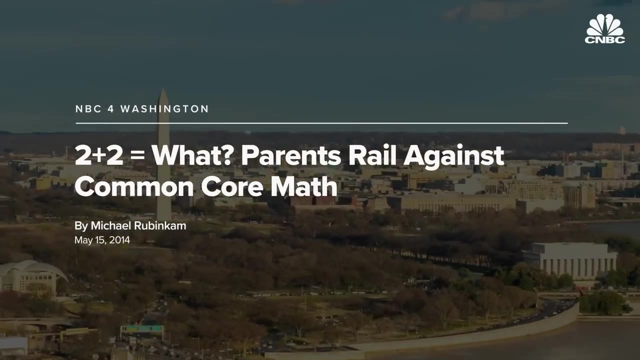 One of the most challenging aspects was we understood that the curriculum was not the same as the traditional curriculum. We didn't do anything but write all the successful and the bad and the horrible. We learned that our families were discriminated against. We learned that our parents, our kids, our 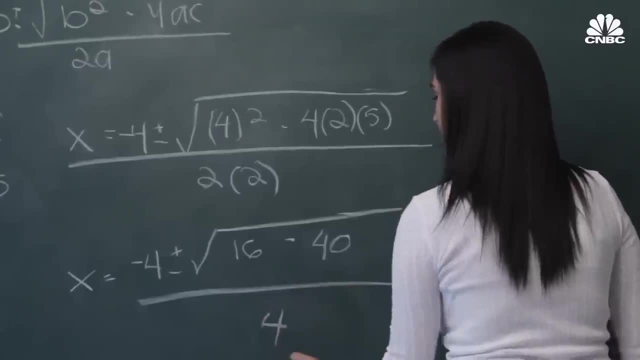 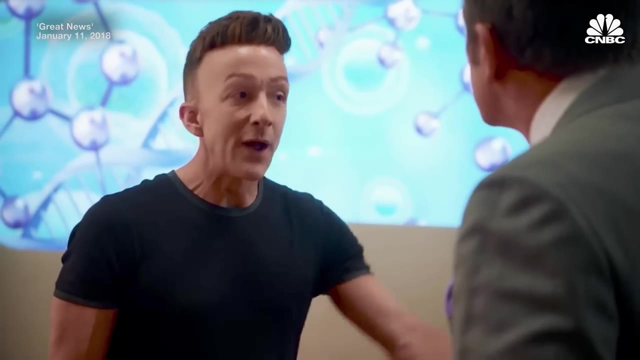 children were discriminated against because they were not expected to go to school, and we were basically thrown a curveball into what it was and had to really adopt new practices. But a couple of years after its launch, it was met with confusion and ridicule.